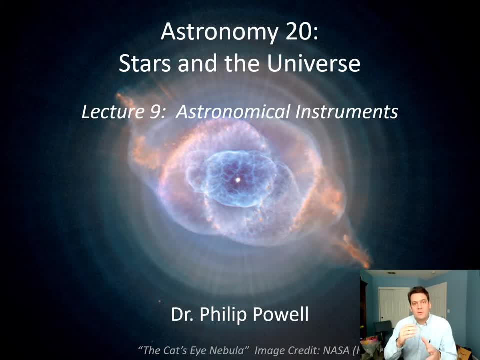 Today we've come very near the end of the introductory third or so of the course, As we talk about astronomical instruments- which is a fancy way of saying- mostly telescopes. Once we do that, then we'll be in a place to actually take the next step into analyzing starlight, which will form the majority of the next three lectures. 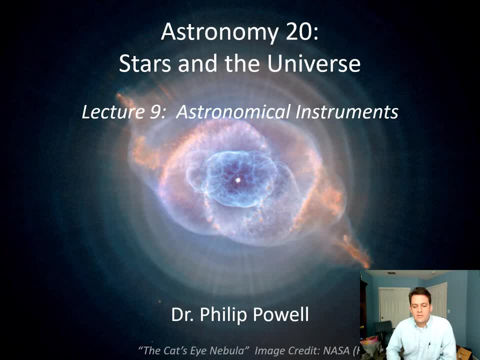 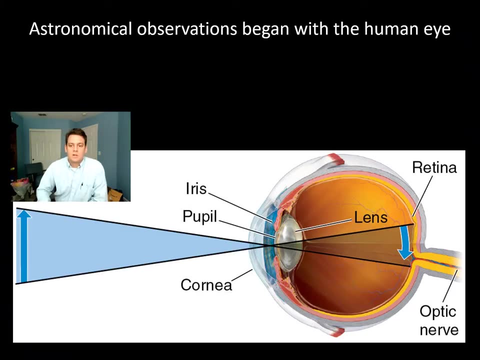 And that's really where we start squeezing as much information out of the light that we capture as we can. So with that, let's go ahead and jump in. So if you remember- and I keep referring to this- But in the very first lecture I made the claim that astronomy could be argued to be the oldest science. 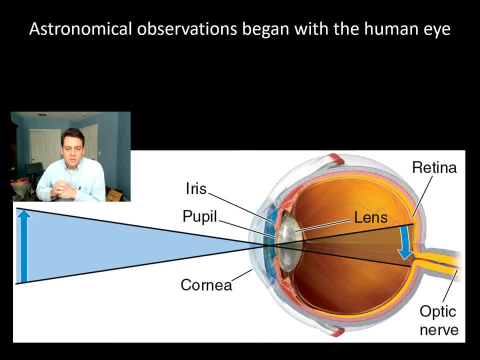 And the reason is that all it takes is your eye to make observations And, as is fairly obvious, for the vast majority of human history, the human eye is the only observational piece of equipment, if you will- that astronomers had at their disposal. 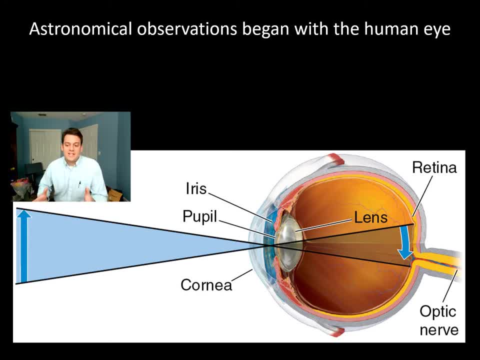 So we're not going to. this is not a class on human anatomy, But it actually is helpful to at least look at the background, The basic anatomy of the eye, because it turns out that, as we, throughout history, starting in the 17th century and then on to today and beyond, 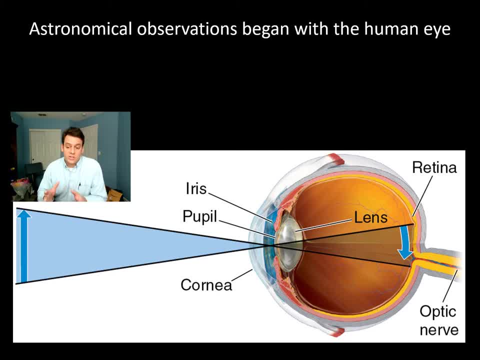 the development of telescopes uses this as its template, And so if you look at sort of the main components of the eye, what we're going to be focused mostly on is the lens here, which is the focusing piece of the eye, And of course there are others. 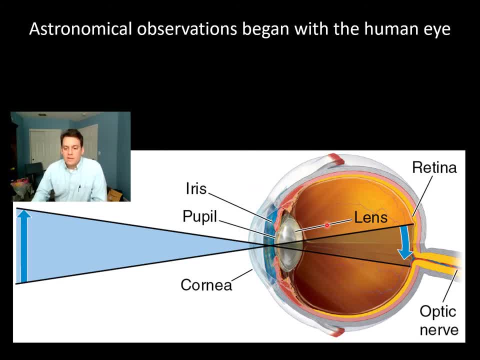 The iris, the pupil and the cornea, and then the retina at the back of the eye, which is sort of where the image gets projected onto. And so, as I said for every, for both the most rudimentary telescopes and the, you know, most impressive modern telescopes, they all have analogies to these, with some caveat with regards to the lens. 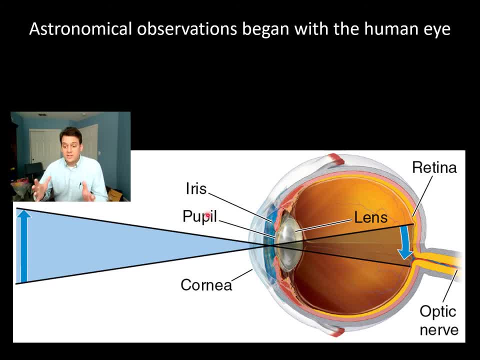 And we'll say more about that coming forward. So, anyway, this is the iris. It's the oldest telescope, if you will, You know it's the one God gave you And you know light comes in through the pupil. 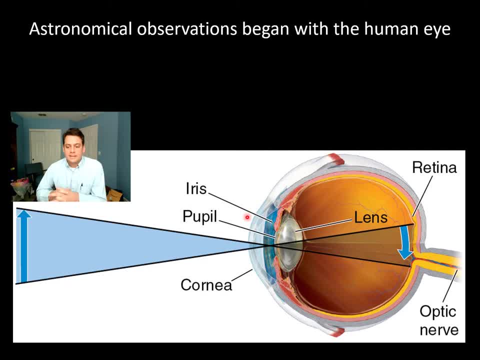 So the pupil is what we'll very often call the aperture, which just means it's the opening, It's where the light comes through, And then, in the case of the eye, it is focused by the lens. So the rays of light that enter the eye are bent by the lens in a process, through a process that we'll talk about in a little bit. 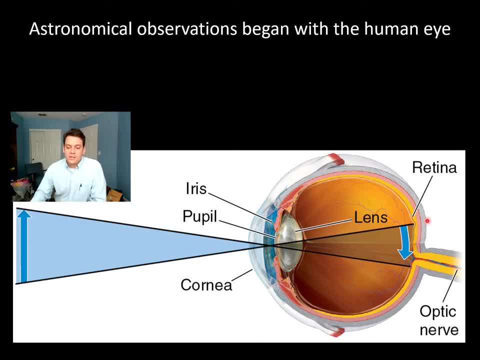 And then, as is noticed here or as is denoted, it's the eye And, as is noted here and is worth mentioning, the image. you know, the arrow here on the left, which is the object you know that you're looking at, is right side up. 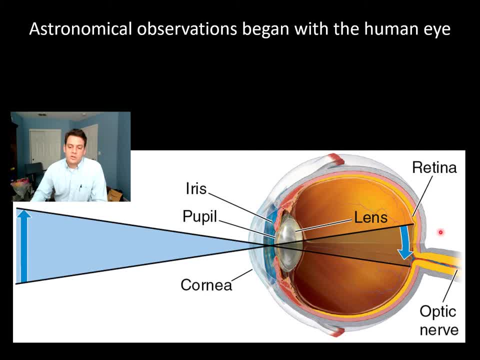 You know, the arrow is pointing up, whereas the image as it's projected onto the retina is actually upside down. And that's true. It turns out that your eye, or your brain, flips that back around for you. So in your perception, you know, we perceive things properly. 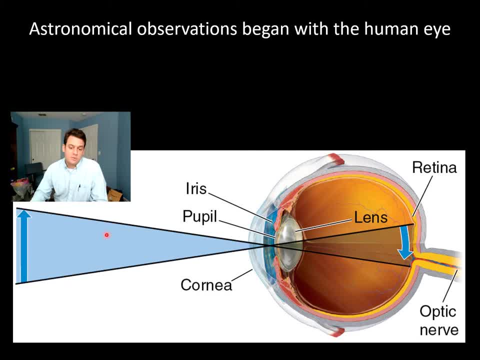 But it is the case that it gets flipped upside down here, You know, just Because of the way that the light rays are bent through the lens. So, anyway, that's the oldest piece of observational equipment for astronomers. Now, I've made this comment before and the precise numbers that are quoted here will be different from, you know, one book or set of slides, one lecture or two, another. 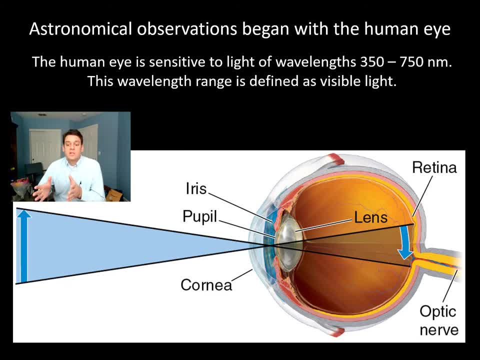 But the human eye is sensitive to lights of a particular wavelength And sometimes you'll hear those quoted as between 400 and 700 nanometers. Here you know, I say 350 to 750.. The reality is that different people's eyes have slightly different sensitivities. 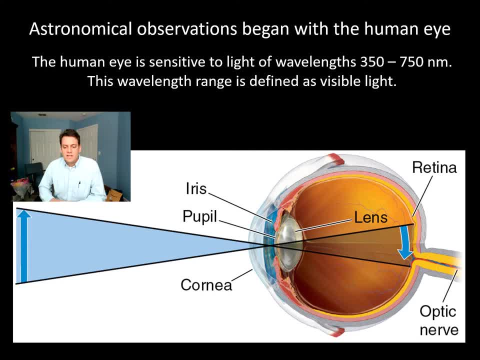 And so some people will be able to see something that others will not. It's kind of a fuzzy range when you Fuzzy cutoff when you get to either end of the range, But it's a particular range of wavelengths that define visible light. 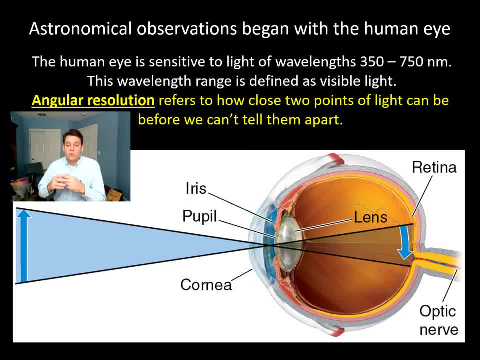 Okay, So we can only see. you know there is light, as we've talked about in the conversation. So we can only see light in the context of spectra. There's all There's. you know an infinite number of wavelengths outside, either at higher wavelengths or lower wavelengths outside of visible range. 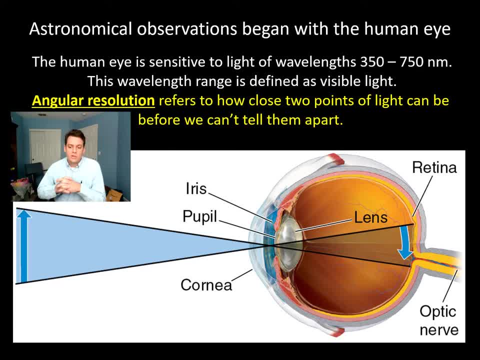 And now we know how to you know, we build telescopes to capture those And we can actually learn a lot about things outside or out there, from light, that's outside the visible range, But certainly historically, before you know, advanced technology came along. 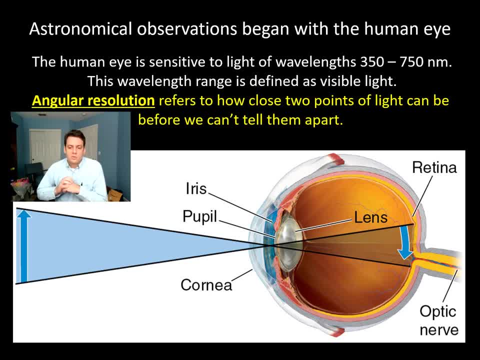 we were stuck just making observations with our eyes. We weren't restricted to studying those, you know, those wavelengths that were, in fact, visible. To introduce a term that we're going to be using, angular resolution is a term that means how close can things be before they sort of merge together, right? 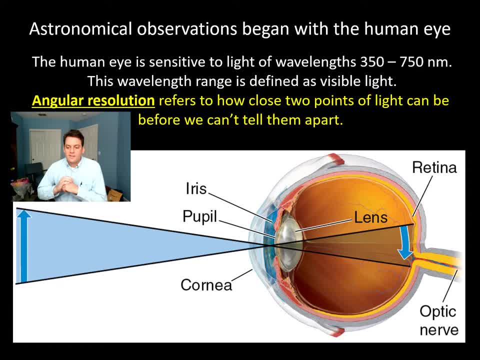 So if you imagine, if you have two points you know, say, a foot apart, that are a foot away from you, you can easily tell those points apart. But if these same two points are a foot apart and you move them a mile away, 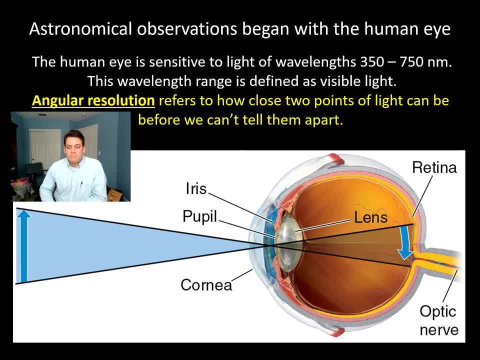 and you move them a mile away away. now you're not going to be able to see them apart anymore, right And so, and we'll have some more examples here. but the angular resolution means what is the minimum angle between two objects that you're viewing which you can tell apart? Because, obviously, if they're very far, 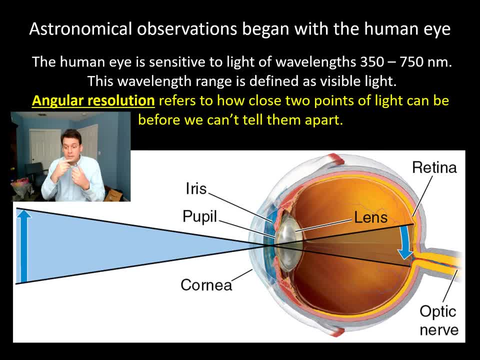 apart angularly. you know, if they're 45 degrees apart, as viewed from your vantage point, then they're very easy to tell apart, But the closer they get, the harder it is, and at some point you can't tell them apart anymore, And so that angular resolution is something that we're going. 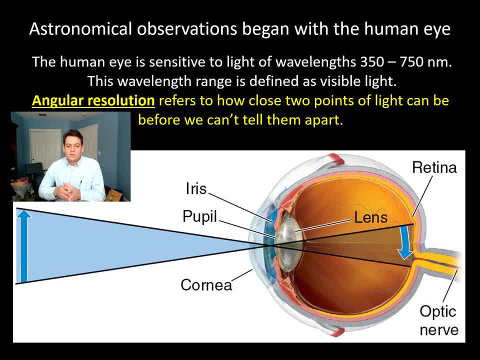 to refer to a lot today, because it's sort of the defining characteristic of how good a telescope is, or it's one of the defining characteristics: The higher angular resolution is, you know, the better the telescope is right, Because you can see better. And so if you have very good vision, 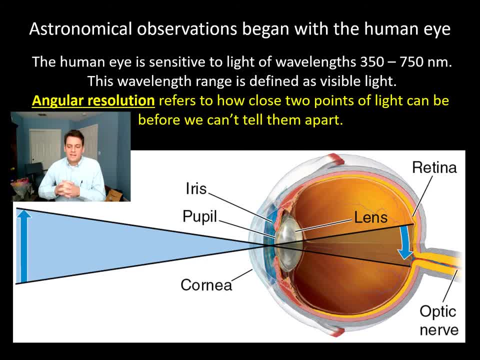 then you can resolve things well, And if not, then you can't. So for the human eye, the angular resolution is limited by the size of the pupil, And the pupil, again, is just, you know, is the aperture of the eye. It's the hole through which light comes in. 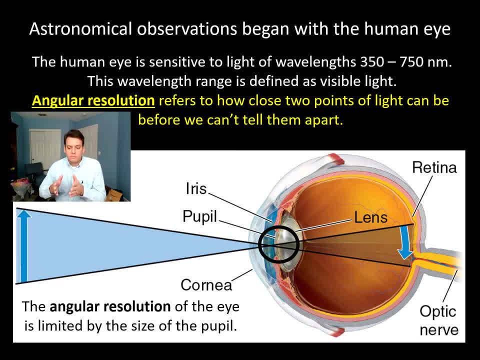 And so the smaller the hole is, the lower the resolution. The larger the hole is, the bigger the resolution, And this is something that we're going to come back to again and again, again, in the context of developing bigger, better telescopes, because the larger the aperture is, the more light you can get in. 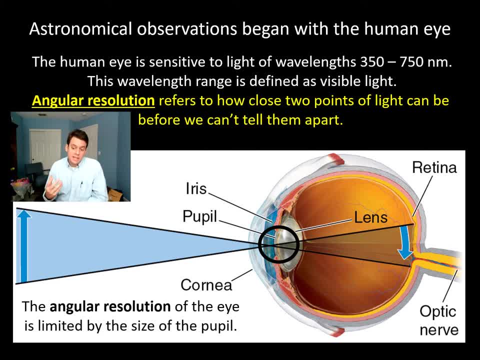 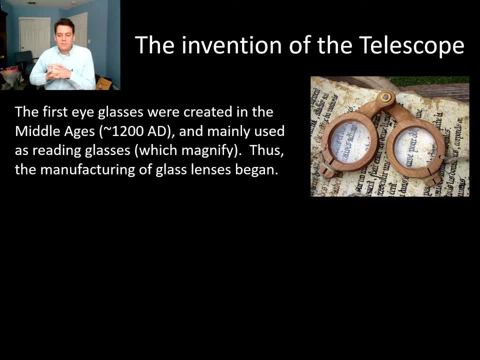 the better resolution you can get, the better images you can get and the more information you can get. So the telescope, you know, is without doubt the most important piece of astronomical stuff. right, It's the most important apparatus ever developed in the context of astronomy. 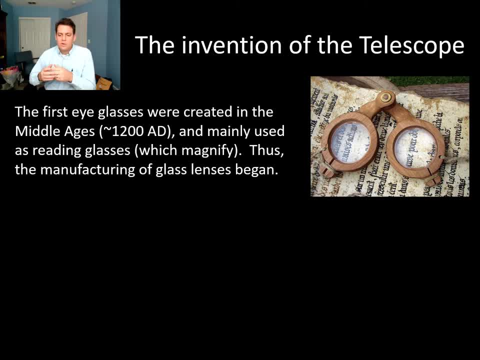 And we've talked about it a little bit, but they kind of came on it that they were. you know, it didn't come out of thin air. right Eyeglasses, for example, were created first, around 1200 AD. so you know- and this was something before I taught this class- 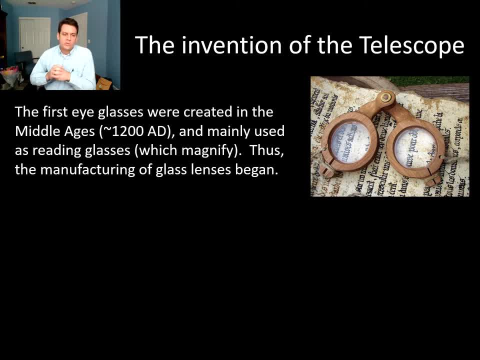 I had no idea they had been around so long, And they were mostly used as reading glasses, just as magnifying glasses, basically. People realized that hey, if you curve glass in a particular way, you can make things look bigger, And so 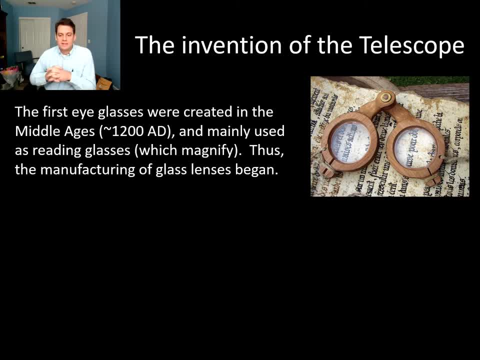 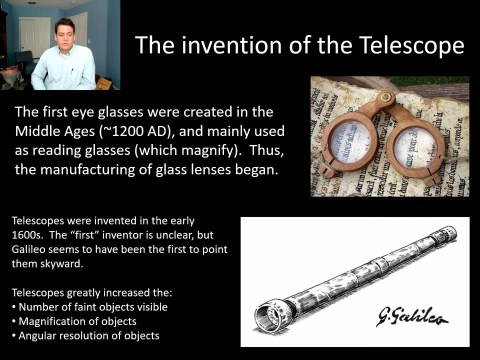 so reading glasses started to be a thing Almost a thousand years ago, And it's impressive to me that they were able to grind lenses smoothly and actually accomplish that. Obviously, that technology improved over time, But it took several hundred more years before it occurred to anyone you know to use this technology. 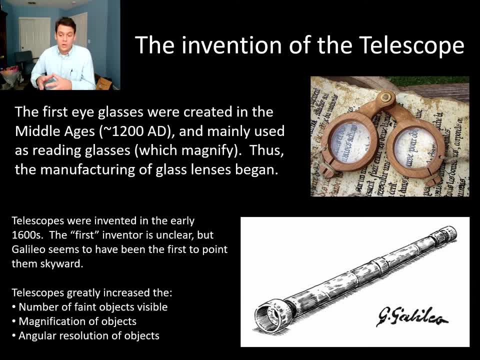 which basically already existed, at least in part, in the context of glasses, and apply that to the sky. Now you will very often hear- and you will probably even hear me say this a couple of times during the course, though I try to caveat it a little bit- 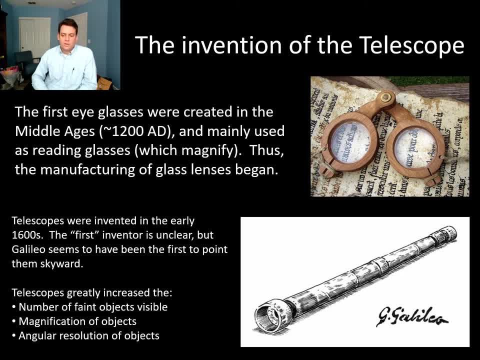 you'll very often hear Galileo credited with the invention of the telescope, And there probably is a sense in which that's true. There may be a sense in which it's not true, but the reality is that there were a couple of different people in the early 1600s. 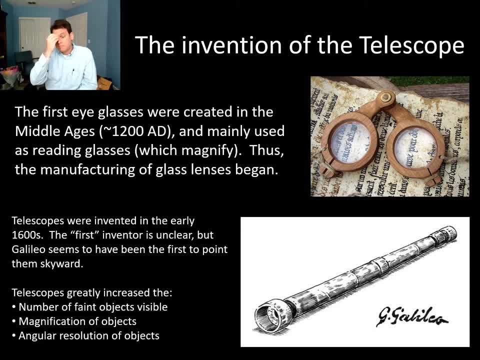 first decade of the 1600s that did very similar things. There is no question that the technology that was in the earliest telescope that Galileo used was not developed by him. So the technology itself was not developed by him. In fact, what became telescopes and what Galileo used was first used on the sea. 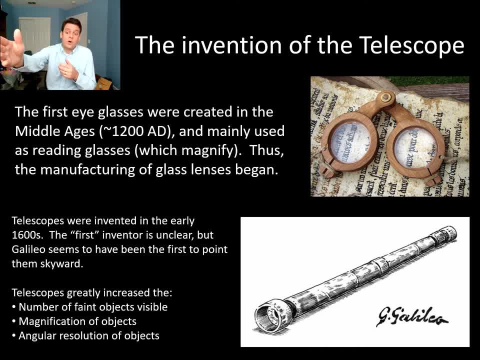 It was used by ship captains so that they could see out farther and maybe tell if they see a spot on the horizon. you know a ship coming and they want to see: is this friend or foe? is this a pirate ship, or is this, you know, another merchant ship? so on. 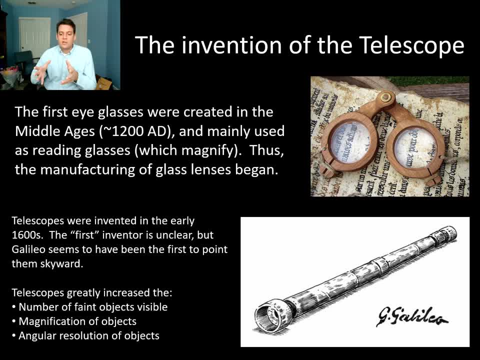 Well, and certainly you can see land more easily as well. So you can see there are a number of applications for these magnifying objects or devices in the context of shipping. But Galileo had the good sense to just take that and point it up. 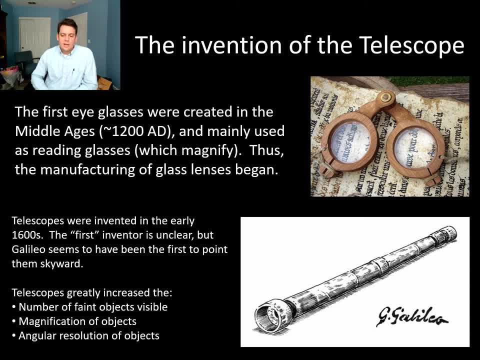 And so that's the extent to which he invented the telescope. But certainly, once he recognized the value, the value of that of telescopes, he certainly started developing his own, He built his own and he took it and ran, as it were. 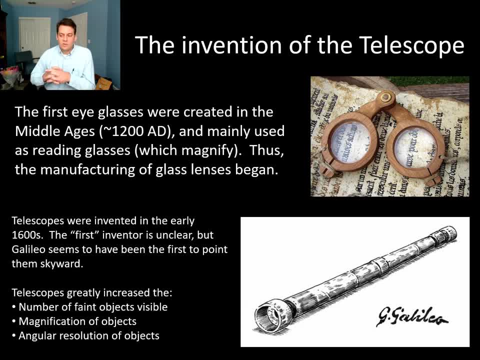 And they did three particular things that were just sort of, you know, mind-boggling in terms of the advances that they made, even with the relatively rudimentary technology they had at the time. The first is that the number of faint objects that were visible just exploded. 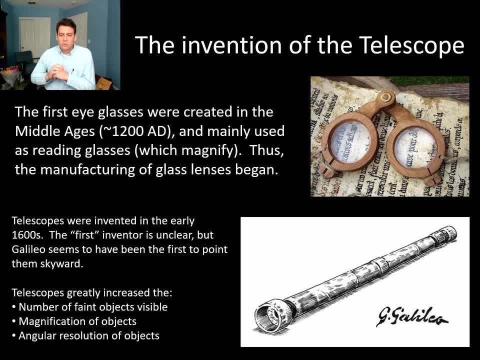 So you know, if you go outside on a dark night, you know you look up, you see there are a lot of stars, but there's a lot of empty space too. You know a lot of just blackness in the night sky. 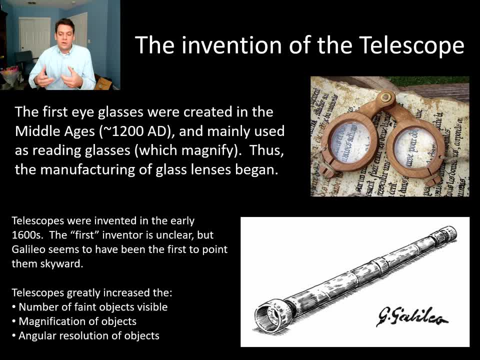 When you look through a telescope. Galileo immediately discovered that there were a whole heck of a lot of other things that were just too faint for him to see with the naked eye, But with the magnification provided by the telescope he was able to see a lot more. 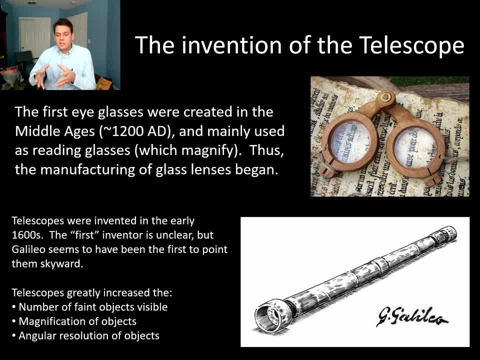 So that's the first thing. The second thing is that those objects that he could see, even those that he could see with the naked eye, were bigger Right, And that's one of the one of the big advantages of a telescope. 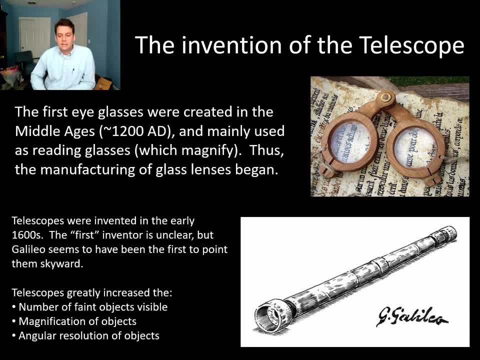 is? it just makes things bigger so that you can see detail in a lot. you can see a lot more detail. And then, finally, the angular resolution of the objects increased. So again, he was able to distinguish between things that to the naked eye were indistinguishable. 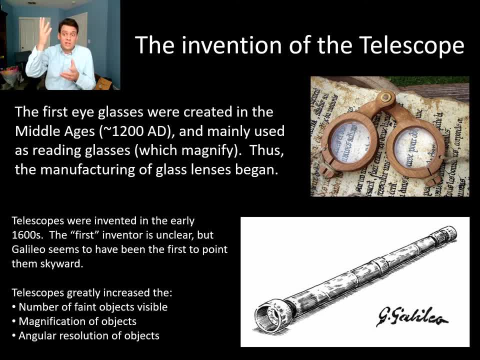 So you might just see. for example, you might look up and see a dot of light in the sky and say, ah, there's a star, I'd like to see that a little better. You look in through the telescope and you see. 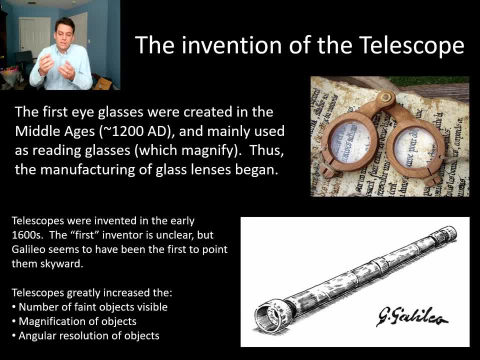 in fact these are two stars, or even three stars that are very near each other as viewed from the Earth, But with the eye they can't be resolved, whereas with the magnification and the improved angular resolution provided by the, by the telescope, 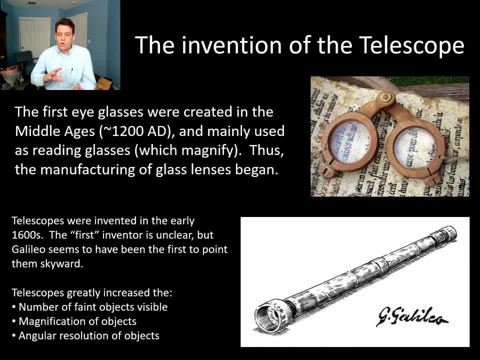 you can, And so these were three things that just you know. it was like flipping a switch in terms of his ability to see things. You know, astronomy had been around for a long, long time, obviously, in terms of observations made around the world by 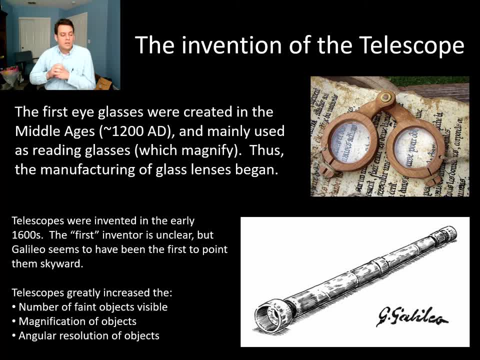 by, by ancient culture, that that we know about, But none of them could. all of a sudden, Galileo was the first and the only person in human history to be able to see all of these new things, And so it was a great time to be him, because anywhere that he pointed, the telescope 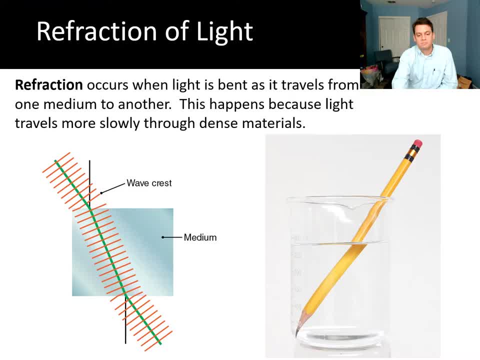 he's going to discover something new Now. the early telescopes used lenses, as I mentioned, and we'll say more about the lenses and and other ways to to construct telescopes, But but certainly lenses were the first, first main component. 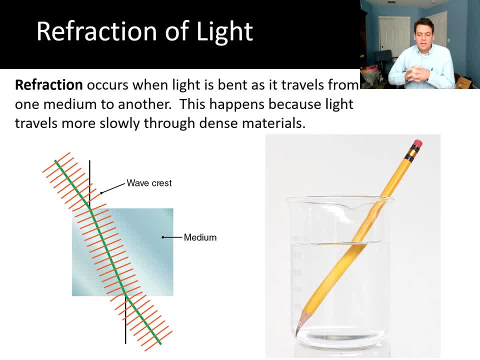 the key component of the earliest telescopes, And those lenses were made of glass and they bend light using a property known as refraction, And refraction, it turns out, is a property of every kind of way, So sound waves refract. 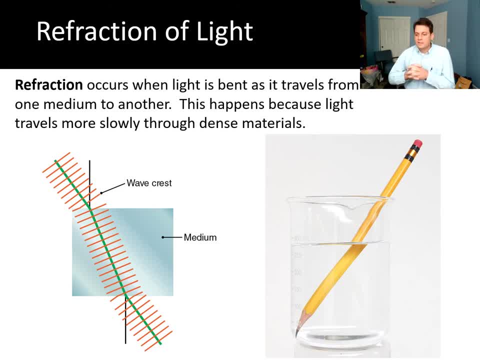 light waves obviously refract water waves refract, And refraction is just a fancy word. that means waves bend, they change directions when they move from one material into another, And we very often will refer to materials as media, You know. 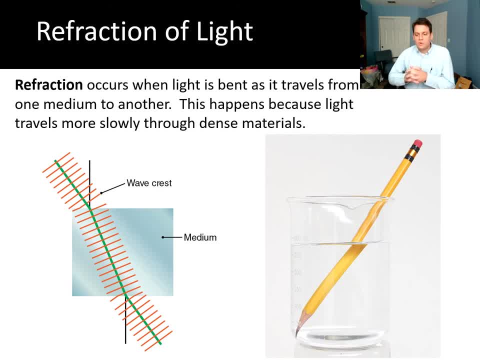 medium is the singular, media is the plural. So when a when a wave moves from one medium to another, it will bend. How much it will bend will depend upon the speed of the wave in in those two different materials. If this were a physics class, 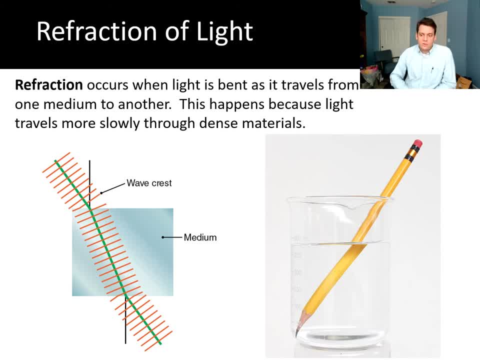 we would spend some time on the details. You know that turns out. there's a mathematical equation, known as Snell's law, which relates the the angle of incidence to the angle of refraction, And you can actually calculate exactly, you know. 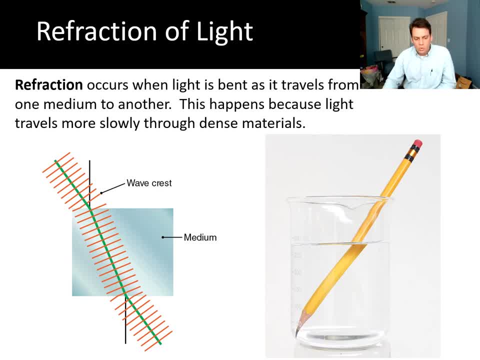 how, how the waves will bend For us. right now, we're going to focus on the, on the qualitative aspects, And so you know we'll very often- well, to the extent that we do this, we're not going to draw a whole lot of. 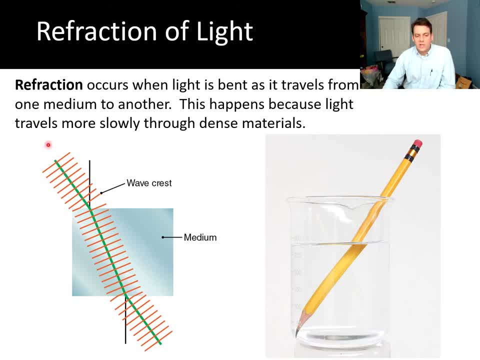 of pictures like this. But but what's being shown here is that the green represents, you know, a beam of light, And these red lines which are perpendicular to that beam are known as wave, wave fronts or wave crests. 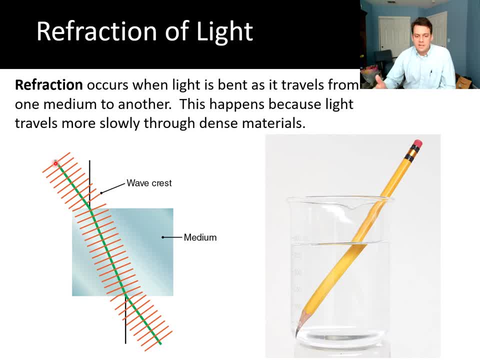 You could think about it as being the peaks of of this wave. So this is, you know, a sinusoidal wave, you know, with peaks and troughs. You can think about these red lines as as denoting where the peaks are. 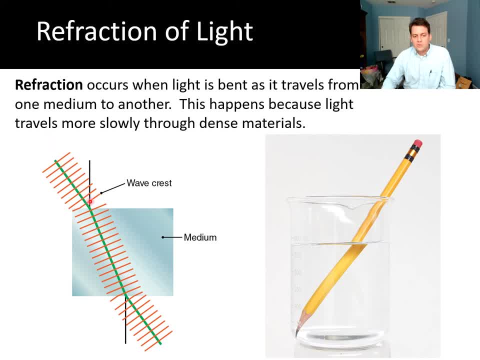 And so the the wave is traveling from air into glass and it bends then as it enters, And then it bends, and then it bends again when it, when it exits. And one way to think about this: why this would happen. 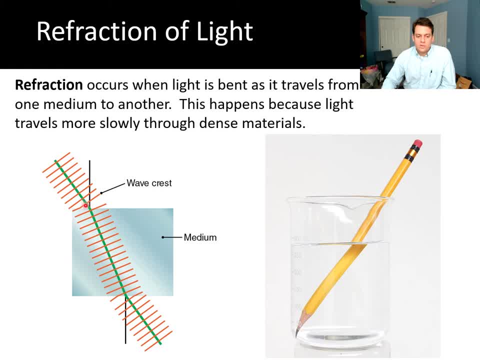 you know, is just that as the wave front enters the, the new medium, as it moves from one medium to another part of the wave front, enters the glass first right, Unless unless the light gray is moving exactly perpendicularly to the surface. 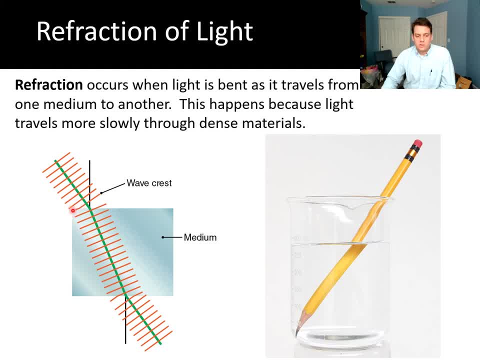 part of that, and in this case, you know the the left part of the wave front will enter the glass first, Before the right part of the wave front, And that's important because it turns out that the speed of light is lower in glass than it is in air. 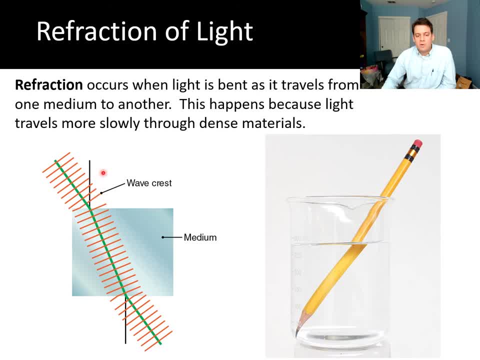 And so, as a result, the the right part of the wave crest is moving faster now than the left part, because the left part is in the glass and the right part is still in the air, And so the result is that the wave front bends. 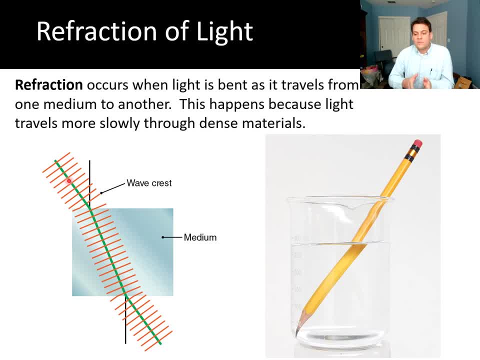 It's a lot like driving a car. you know one of your tires ends up in mud and the other part is still on on a paved street. right, You're going to end up turning towards the mud because the your tire that's in the mud is not going to be able to travel as easily. 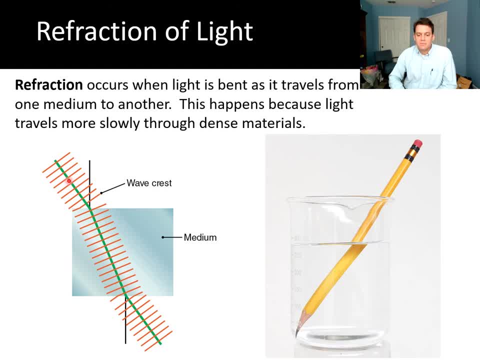 And so it's exactly the same. you know basic mechanism that that happens here And it gives rise to some very useful results that we're going to: the Galileo captured and exploited and many others after him. And it also does some funny things, just like: 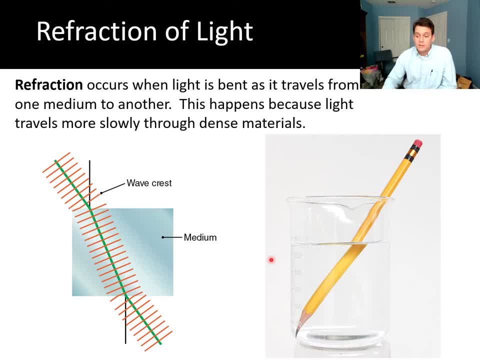 you know, making the pencil appear broken because the light is bending as it comes through the water or as it leaves the water and enters the air. the light is refracted, it bends And so it turns out your brain when, when we decide where an object is. 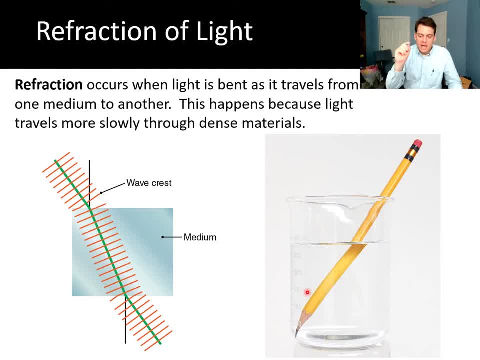 we basically track the light rays back backwards in a straight line. Okay, Because our brain knows that light travels in a straight line, unless it doesn't, And it doesn't when it bends coming out of a medium. uh, and so you can spend. 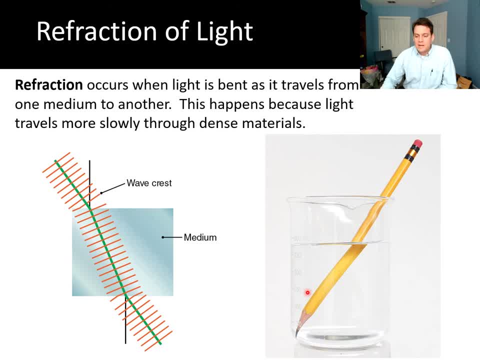 uh, we can spend more time talking about that particular uh phenomenon, but but the basic mechanism is just what I've said: When waves, when any waves- and for us light changes, media moves from one material to another. 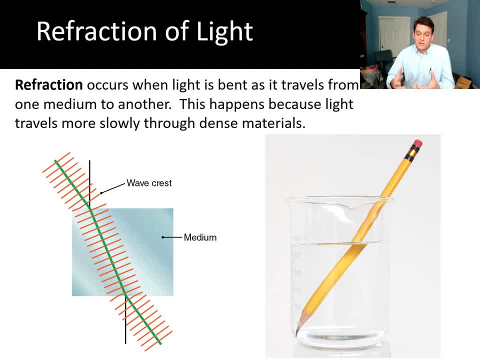 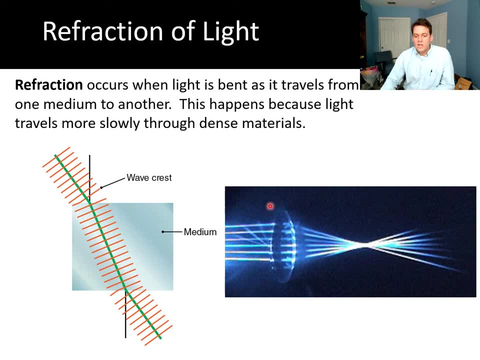 it will bend, Um, and, and it will bend by a specific amount that we can calculate. And so you know more, more to the point here: if we take a lens like this, um, we, we can focus the light using that lens. 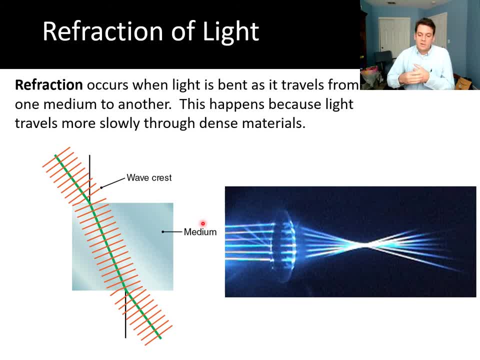 um in a particular way, And so, for example, if we wanted to focus the light in a specific place, um, we could construct a lens to do that Um and and so in this particular case, you can see, you have rays of light that are parallel to one another coming in. 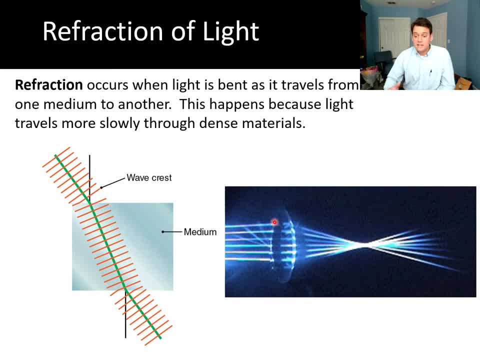 from the left, They all bend. they bend by different amounts depending upon you know where they hit the surface of the of the lens, But then they are all focused down into a point uh, which, not very creatively, is known as the focal point. 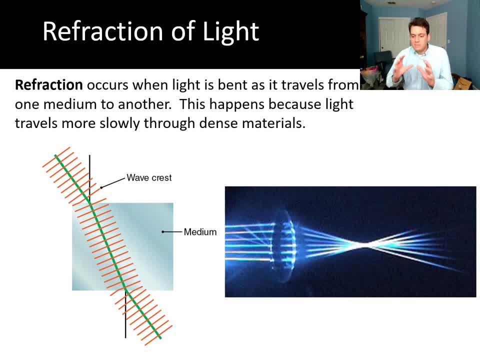 And we'll say more about that, but this is going to be the main feature, this, this is the utility of lenses. This is why lenses are useful, and we'll see the applications, uh, shortly. So there are two main types of telescopes. 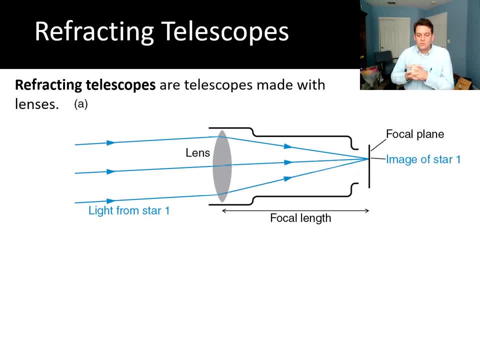 uh, and I sort of alluded to this and we're going to get into into the details now and in what follows. But, uh, the first type of telescopes, uh, that use lenses, are known as refracting telescopes. 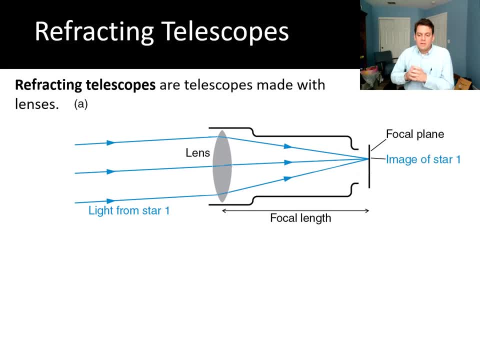 And again, it's not very, a very creative name. Um, they're called refracting telescopes because they use refraction to focus the light. They use they use lenses made of glass to focus the light, And so you know. 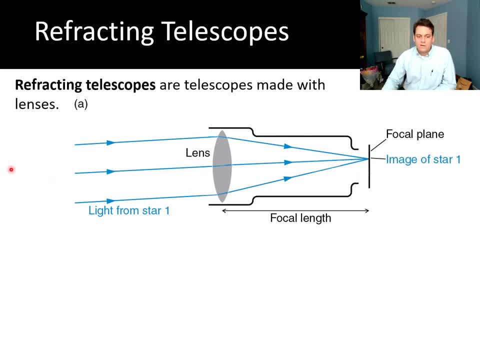 in a not drawn to scale uh schematic. here we have light that will come in from from a very distant star. right. It will come and and those rays will be parallel to one another because they're coming from so far away. 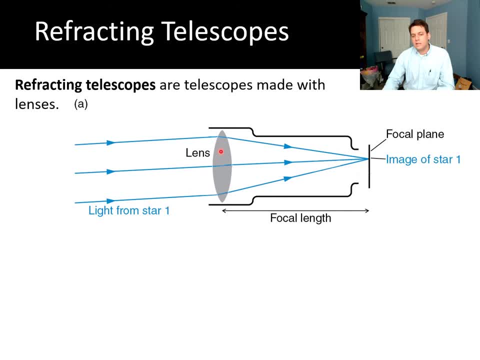 you know they they're going to be parallel rays. They will enter the lens and they will be refracted and they will be focused down to a point or onto a plane that we call the focal plane. And if 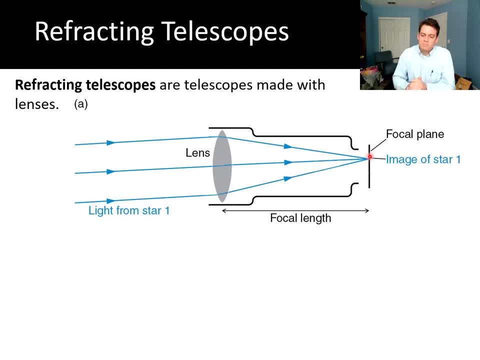 if you, you can imagine having a, a piece of paper there, for example, um, and you would see a dot of of light on that focal plane. that would be the image of the star. Okay, Um, the distance between the lens and the focal plane is called the focal length. 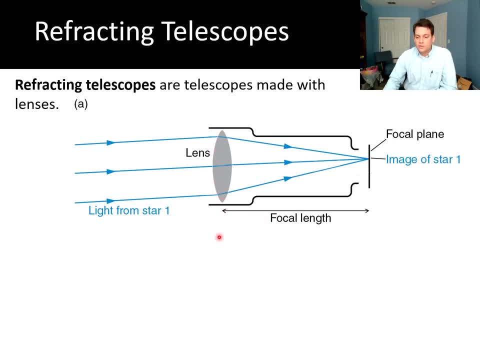 And it it is, uh, determined by the radius of curvature of the lens. So, basically, if you have a very, um, if you have a very big lens with a with small curvature, then the focal length will be long. 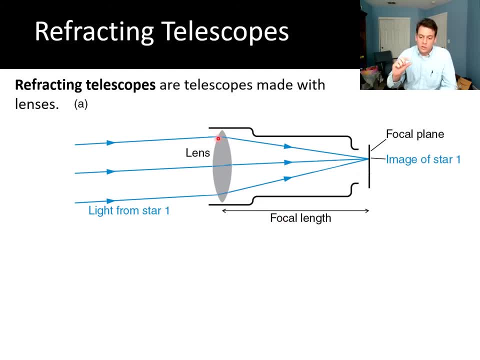 If you have a a smaller lens with a larger or with a smaller radius of curvature um, so it's curved more- then it will bend the light rays um more significantly and the focal length will be smaller. So 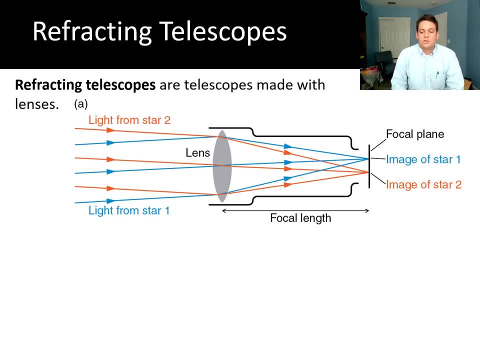 let's complicate things now and add light from a second star. So the second star is somewhere in the sky, but obviously at a different location than the first, And so its rays come to Earth in parallel, you know, as parallel rays as well. 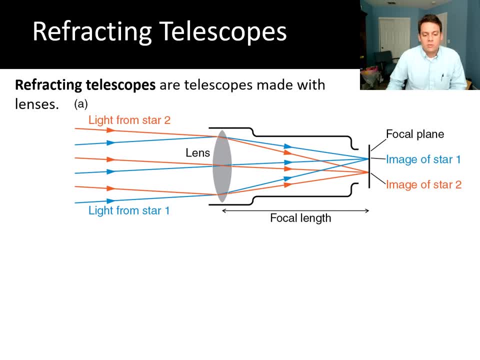 but coming from a different direction, And so you can see that represented here, just because the the orange rays are parallel to one another, but coming from a different location in the sky, So they pass through the same lens and they are similarly refracted. 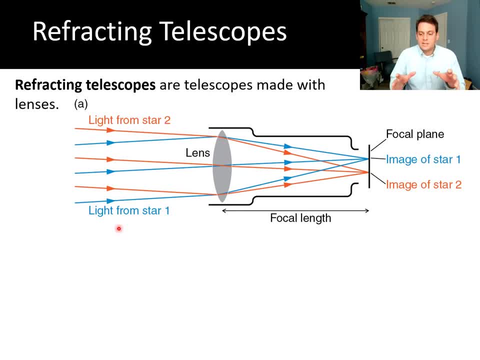 um. moreover, the lens is characterized by its focal length, which is just the. it is what it sounds like. It's the distance over which the light rays are bent enough that they come together to a point Um, and so that focal length is the same. 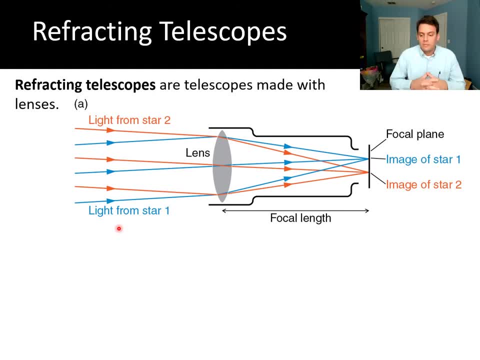 it is again. it's a characteristic of the lens itself, um, and so it doesn't care which image it's forming. All of those images are going to be formed, um, on the same focal length, And so the upshot is that the 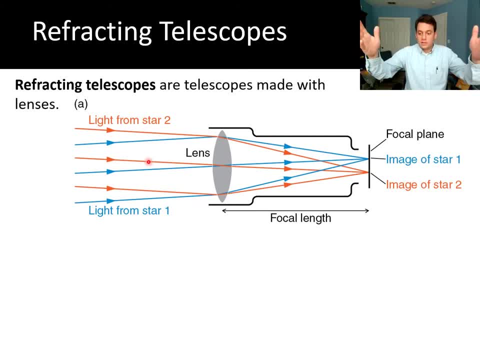 you know, these rays came from two different sets, two different stars in the sky. they're refracted through the same lens and they form images on the same focal plane but obviously in different locations. So you know this is. 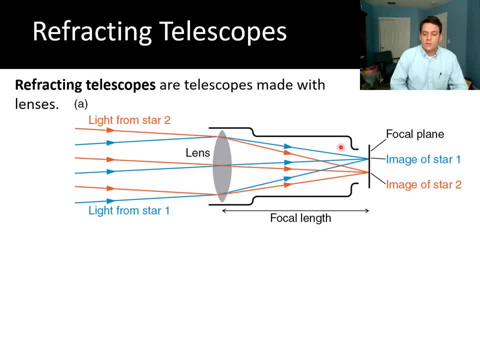 you know it, it starts to get pretty cluttered, even with just uh six rays drawn here. In reality, you've got, you know, hundreds of stars that might be visible in, in, uh, in in a particular. 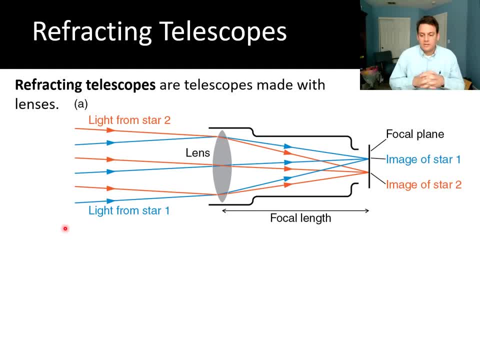 uh, region of the sky, say. And so in reality, that's so. in reality, there are going to be a whole lot of black rays crisscrossing each other, and that's fine. I'm not going to. 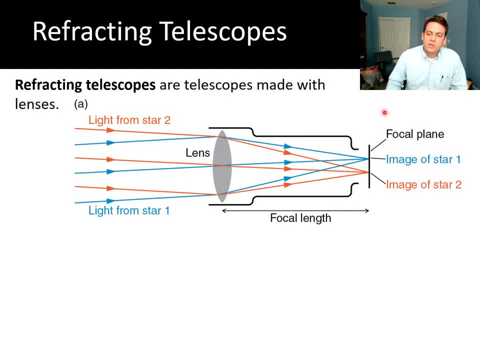 you know not going to make your head hurt by drawing that here, Um, but you're going to have a number of different images. however many stars are out there, you're going to have those images on on the focal plane, Uh. 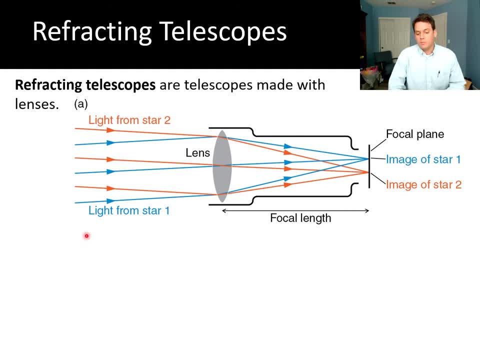 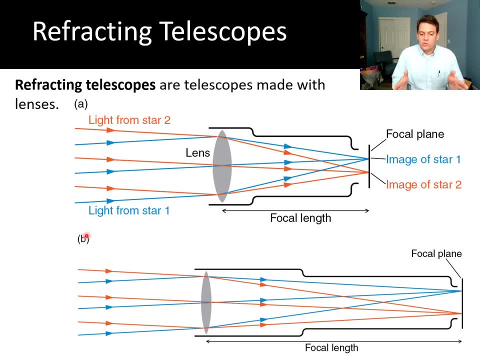 moreover, um, if you have a different telescope with a different focal length, then the you know, the distance over which those rays are are focused, um will be different, And so here, in part B, I've added a. 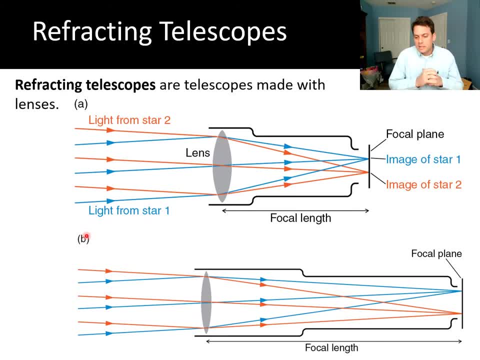 a set of uh. a set of uh. I've added a separate schematic, just with a longer focal length, so you can see, as I mentioned, uh, just a little bit ago, the lens it's, you know. 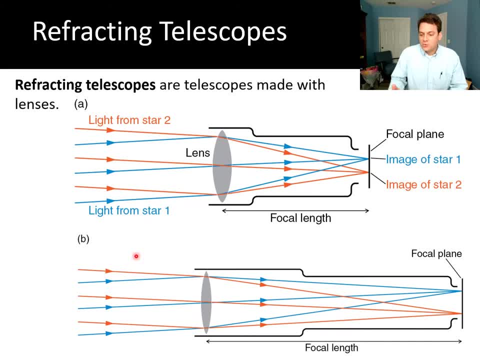 the, the focal length is totally determined by the radius of curvature of the lens. Um, and, as usual, there are mathematical, uh, relationships there, that, uh, that, if this were a course in optics, um, we would, we would dive into. 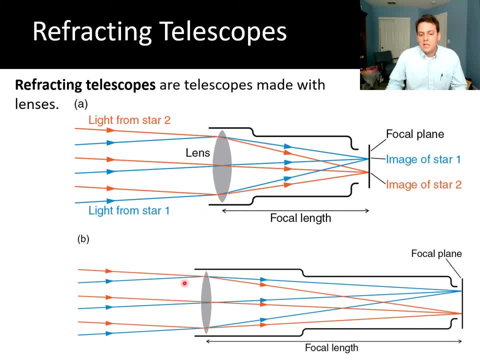 but mercifully we won't do that. But you can see this. uh, in part B the lens has a larger radius of curvature. that, you know, is just a way of saying that if you were to continue this, you know. 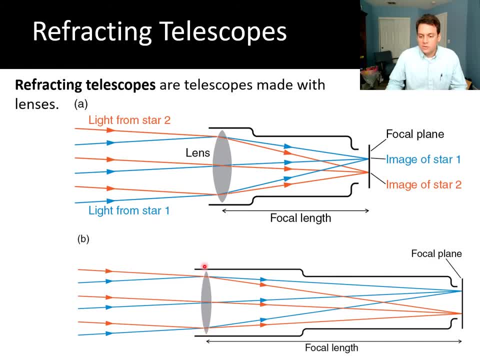 this is uh part of a circle. It's a. it's a circular arc here. So if you were to continue that circle the radius would be a larger in part B than part A. It's not curved as much. 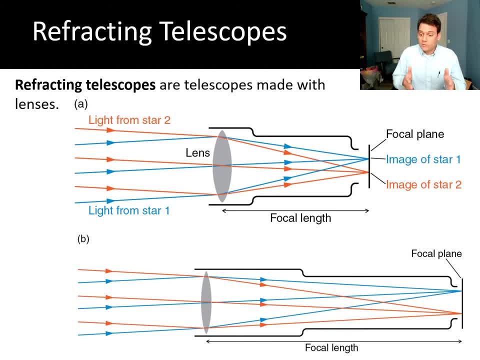 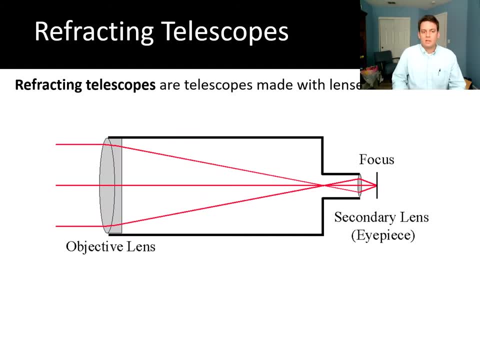 and so it takes a longer focal. it produces a longer focal length. It takes longer for the for those rays to be focused down to a point. So to continue, uh sort of attributes of a refracting telescope, um, refracting telescopes. 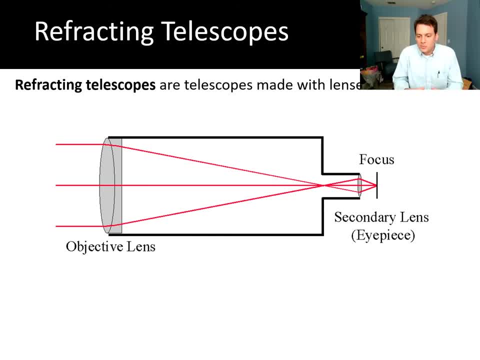 again, just- and I'll say this a few times, just hope, uh, that it sinks in: Refracting telescopes, just by definition, are ones made with lenses, Um, and typically they have two different types of or two different lenses in them. 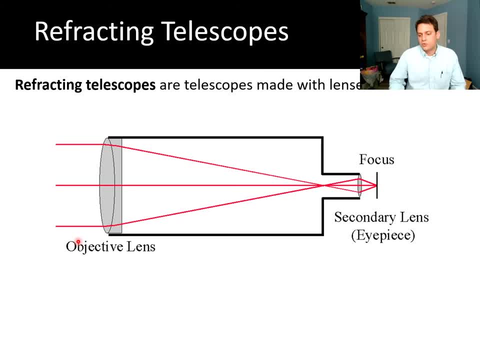 The the first is called the objective lens, and that's the one that we've referred to so far. That's the one through which the rays you know are are focused, And in this schematic you can see that the rays come from some distant object. 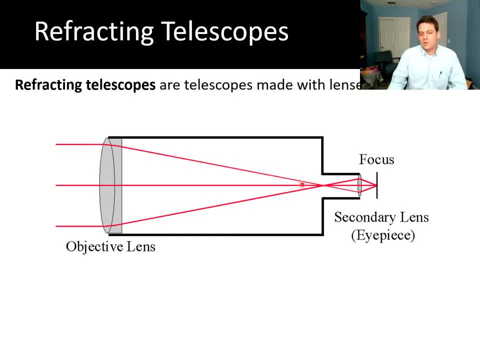 They pass through the objective lens and are focused down to a point here, But then a little bit beyond the focal point. so the rays have have converged, and now they start to diverge again if they continue on past the focal point. 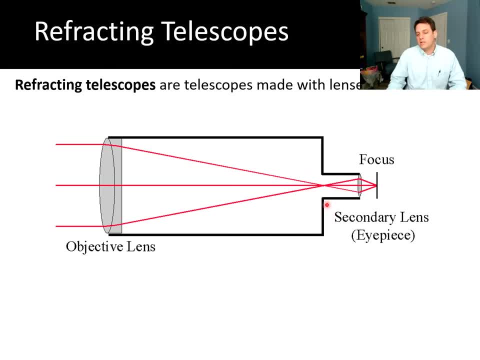 Um, they then pass through what's called a secondary lens, uh, which is in the eyepiece, And then that secondary lens focuses, the refocuses, the light. um, to to a new focus, a new focal plane. 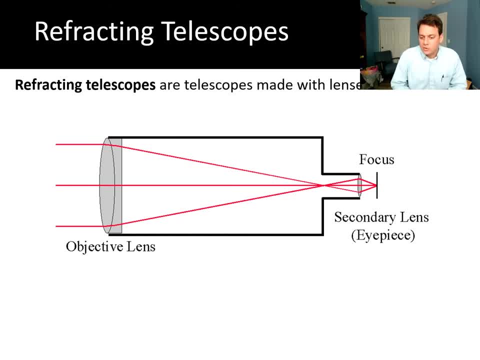 um, which is, uh, hopefully, uh, where you'll put your eye in order to see it. So, telescopes, um, obviously, this is the kind of uh setup that you would have for a backyard telescope, one that 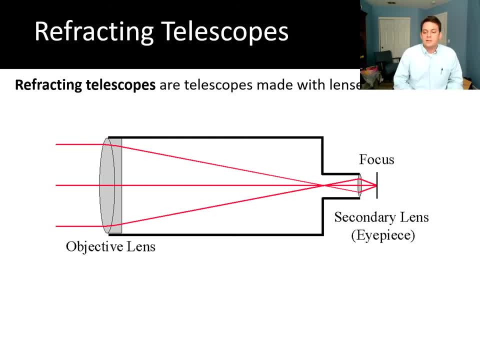 you know that you or I would set up and you'd want to actually go put your eye in it and and look at it. For today's modern telescopes, you know ones that, um, that are used in 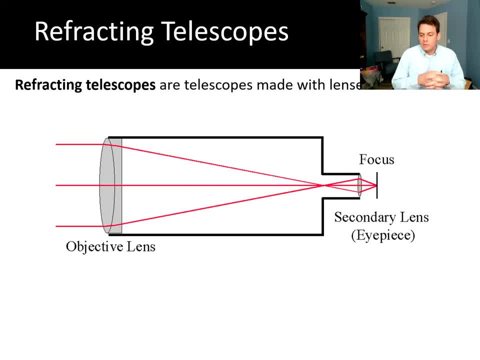 in cutting edge research and so on. uh, they are not ones where people actually put their eyes, you know, up to, And so the secondary lens isn't, isn't necessary. So you know, if you're just going to use a computer to capture the data. 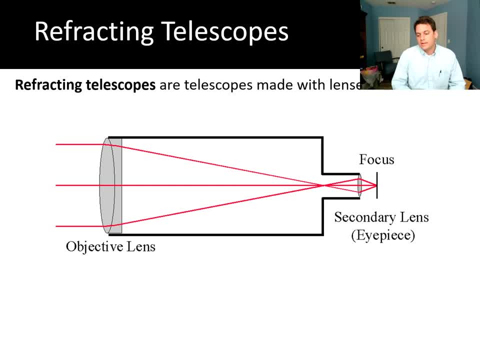 um, and store it and analyze it and so on, um, then you don't need this, this eyepiece, obviously. But but if you, if you want to actually see something and enjoy it yourself, um, you know. 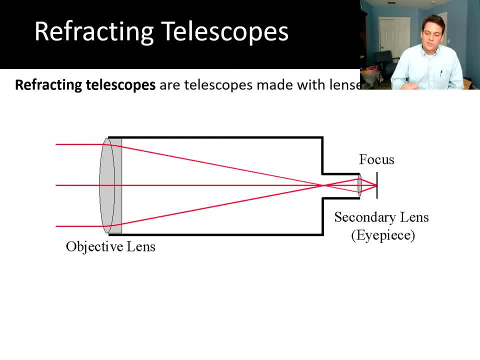 in in real time, then you would want the secondary lens. you know the eye, because that's what you're going to use to to observe. So, as we mentioned in the context of of the pupil and the aperture, 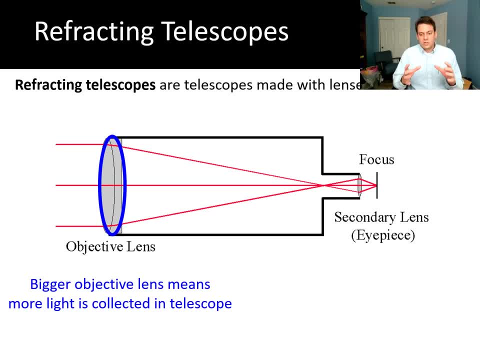 you know the aperture again is just, is the name for the opening through which light is collected, And a bigger aperture slash, a bigger objective lens means more light is collected. right, There's no magic to it. 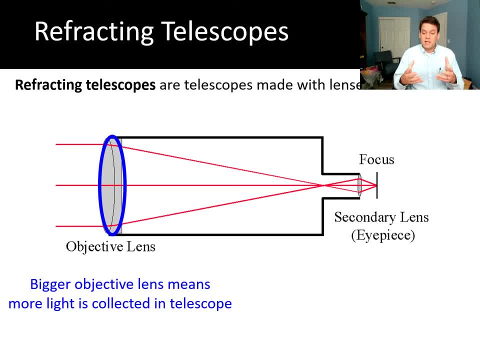 You know, there's some light coming from, from these objects, and the bigger the aperture is, you know, the more light you can collect. So you know, that's that's that's what we're going to do. 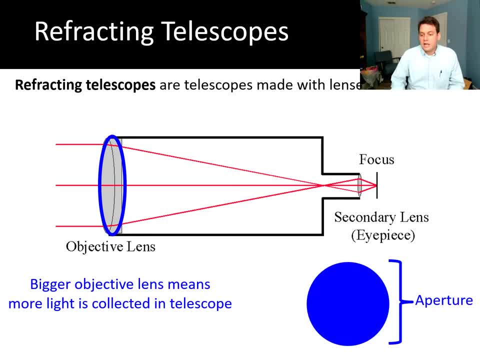 And the aperture is going to be characterized by its diameter, Typically. um. there, you wouldn't need to have a circular aperture, um, but if you had something that wasn't circular, it would introduce, uh, complications that you wouldn't like. 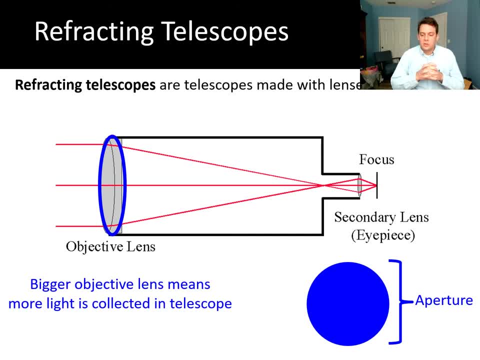 So the apertures that we're going to always talk about are going to be circular, And so you could specify the radius if you wanted, um, but typically the apertures are specified by diameters, And so that's what we're going to do. 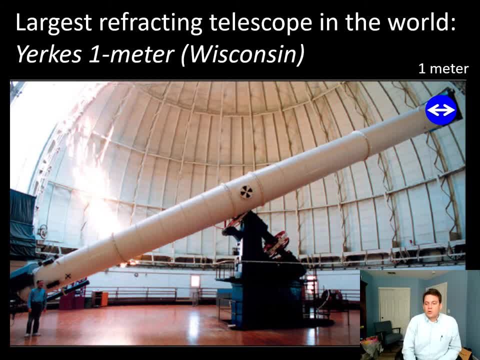 So refracting telescopes, um are what started off the, the astronomical explosion back in the 17th century. Um, and they have have, uh, they've served themselves and they've served us well, Um. the largest refracting telescope in the world is the Yerkes one meter telescope. 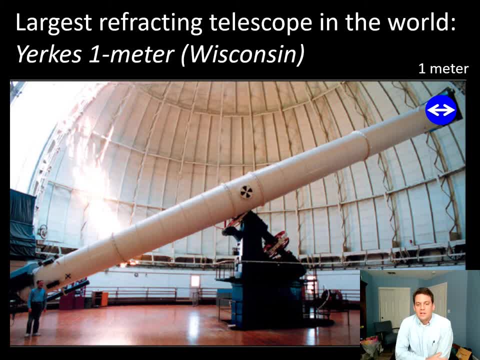 uh, happens to be in Wisconsin. And we, when we say one meter, what we mean is: that is the diameter, that's the aperture, That's the diameter of the light, And, uh, the, the, the, the. 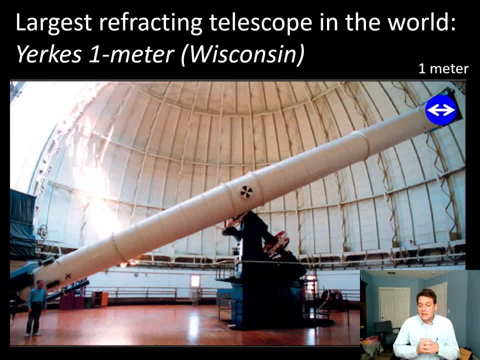 the, the, the. that's the diameter of the lens, So a meter is 39.37 inches, just a little bit over a yard, And so if you can imagine a, a lens which is a yard, 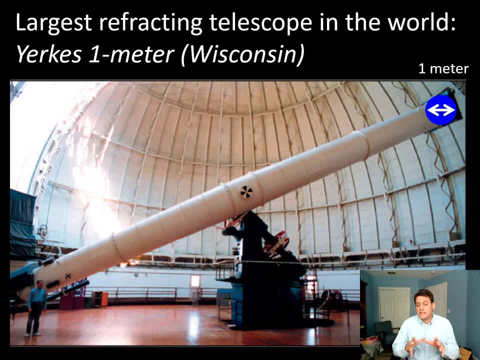 you know, or a meter in diameter, that is a really big piece of glass. And we're going to get to that because it turns out that those, the uh pieces of glass that big are not easy to make. um, in the very 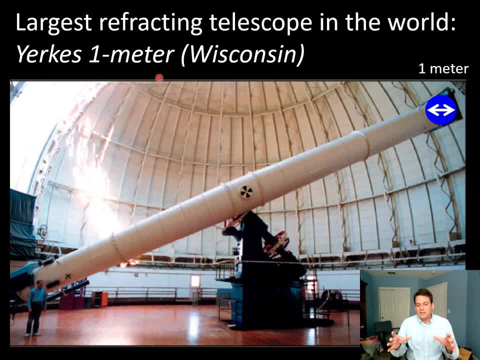 well, you can make a piece of glass that big, but it's hard to make a very high quality piece of glass that big that is good enough to to make good astronomical measurements with, and it's really darn heavy too. I don't know if you think of glass as being dense, but it is, and so 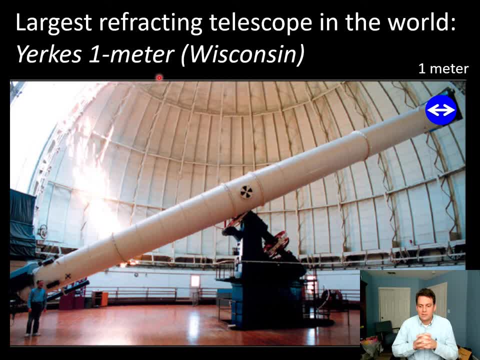 when you have a meter, when you have a, you know, a meter diameter lens, that's a whole lot of weight. but this is a picture of the telescope. unfortunately it is not actually. it still exists, but it is not currently in use, as of last last time that I checked. I think there's some refurbishment that may need to be. 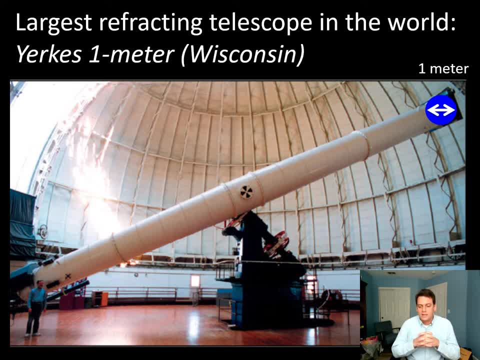 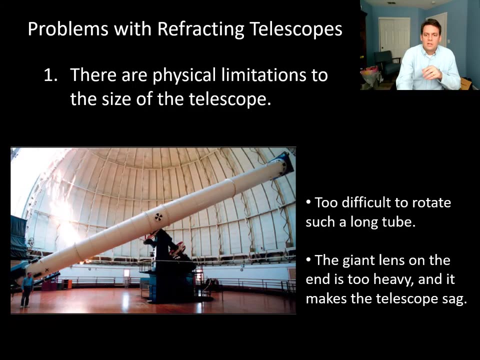 done to the, to the site that it's located at, and and last I saw it was unclear whether that was going to happen. so this is the largest refracting telescope in the world, but I'm afraid it's not being used right now. hopefully it will be again in future. so I haven't said this explicitly yet, but I guess now. 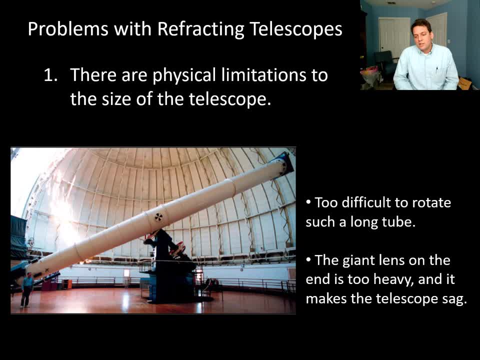 is as good a time as any. but I've alluded to it, refracting telescopes were the first type of telescope, but they are. they are the first type of telescope, but they are the first type of telescope, but they are, as it turns out, not the most common type today, and there are a few reasons. 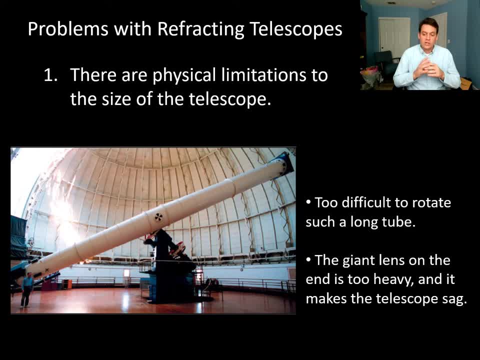 for that. the first I just sort of alluded to, but I'll say it now clearly: there are physical limitations to the size, to how big you can make a refracting telescope, and there are a couple of reasons for that. but one is, remember, the bigger the lens that you make for practical reasons, it tends to. 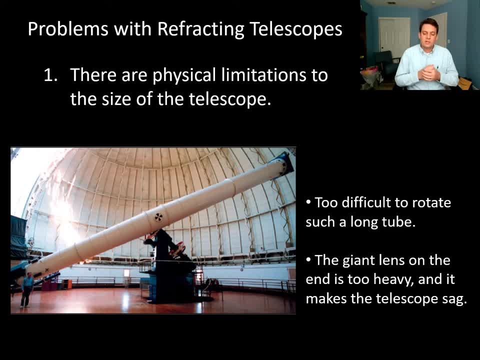 to require larger focal lengths because you can't make it arbitrarily. it's hard enough to make it very large lens. to make a very large lens with a large curvature is even harder, and so you have these large lenses. they tend to require what have long focal lengths, and this is already a 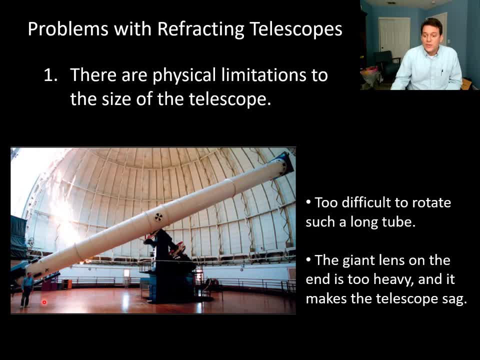 pretty unwieldy focal, you know sort of thing. I mean you look at the focal length here, you know, for scale. there's a guy standing next next to here. he's about six feet tall. I mean you can kind of tell this is, this is a really long tube. 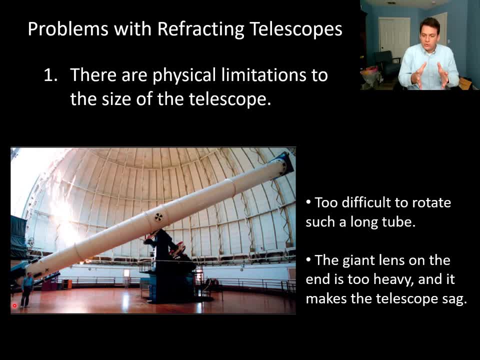 okay, that gets pretty difficult to to move, okay, and just to practically point at anything that you would want to see in the sky. the second thing I've mentioned as well: the lens gets ridiculously heavy, okay, and, as it turns out that it's not just hard to like, mount it up there and put the whole. 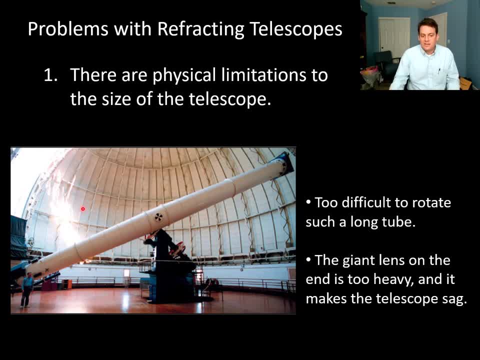 thing together. but now it tends to make the, the steel in the coming- assuming they steal for the two here- eventually gets heavy enough that it it puts undue strain on the steel and will actually make it fail over time and so just practically there really are limitations and the your keys telescope basically. 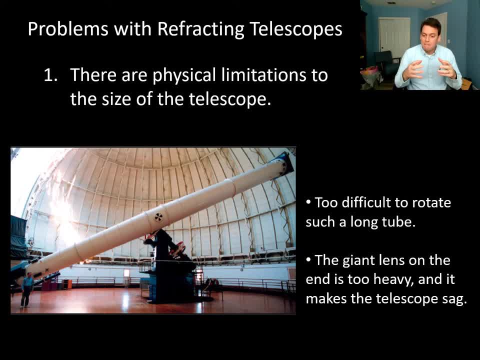 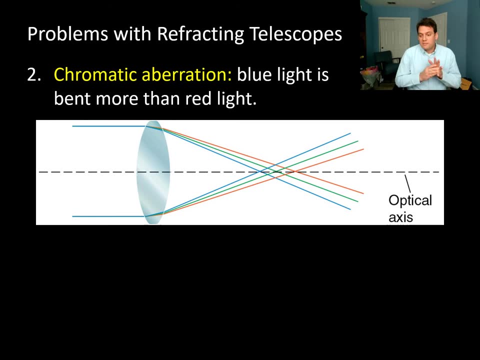 gets to that point in order to make anything bigger. it would be so, so expensive and so difficult to to manage that it just becomes impractical. beyond that, though, there's actually some some physics limitations as well, and in particular, this phenomenon known as chromatic aberration and the the as this schematic 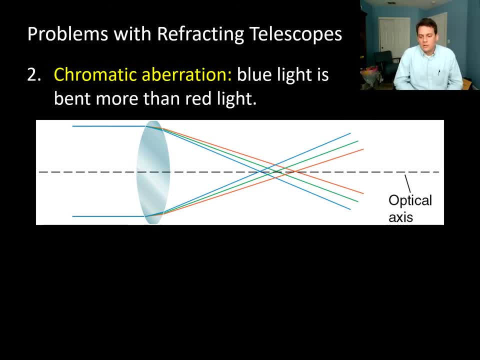 indicates here. the big thing here is that different colors of light are actually refracted at slightly different angles through glass and well through anything, and the reason is that the speed, that the speed of different colors at different wavelengths of light are actually slightly different. in in media, in a vacuum, all wavelengths travel at the 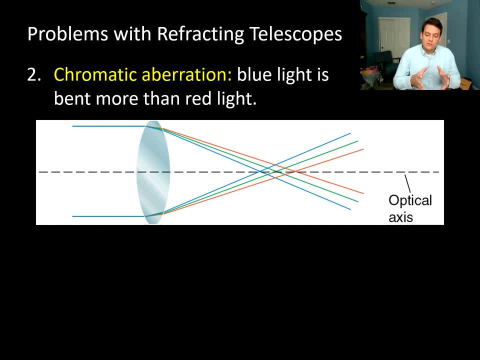 speed of light see, in media they travel very nearly the same, but not quite okay. and so, as a result, the you know, when these rays come in from this distant star, it's going to be a mixture, it's going to be a continuous spectrum in general, and so it's a mixture of all the different wavelengths. but as they 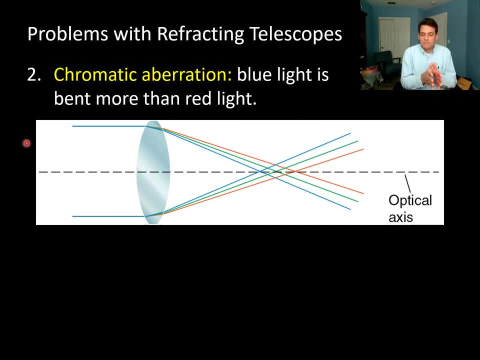 refract through the glass, then those wavelengths get dispersed, they they spread out, and so the result is that what we've so far referred to as a focal point is in fact not a single point anymore, because the blue light has one focal point, the red green light has a different focal point, the red light has a. 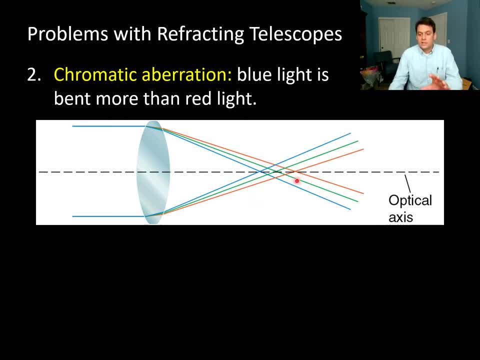 different focal point. now this is not drawn to scale okay, so it's not as bad as what's represented here, but it gets worse and worse as the lenses get bigger, because the bigger the lens is, the larger the longer the focal length, the larger the distance over which these, these rays can diverge from one another. and so, if you 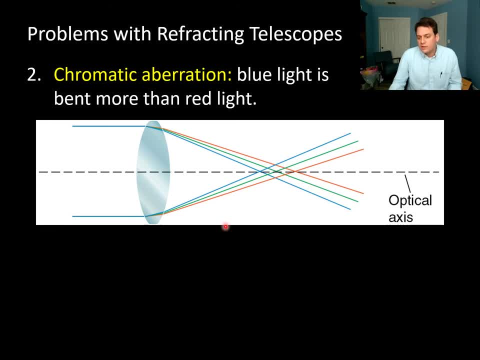 have a small lens, then the difference between the- you know- the blue focal point and the red focal point is so small that you that you know for all practical purposes they're the same. but as you make the lens bigger and the focal length gets larger, now these these different colors focal points end up. 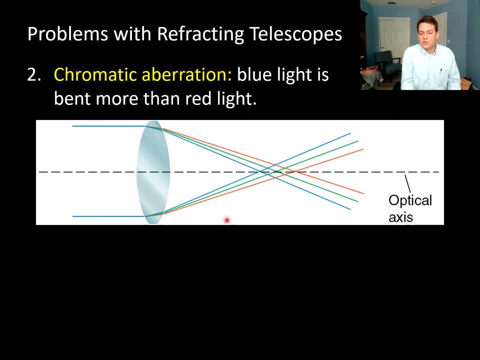 becoming noticeably different, and the result is that the image that you form is skewed in color space, that the colors are not, they're not reflective of the original, of what the star itself is. and so, again, in the spirit of not being created with our naming schemes, we call that chromatic aberration, because you 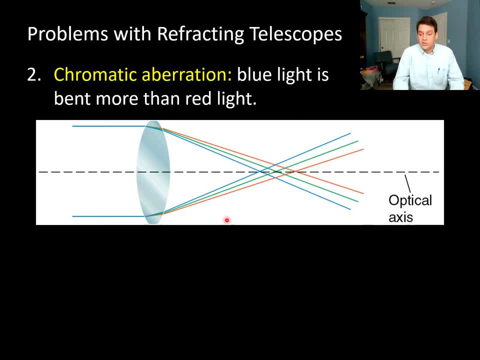 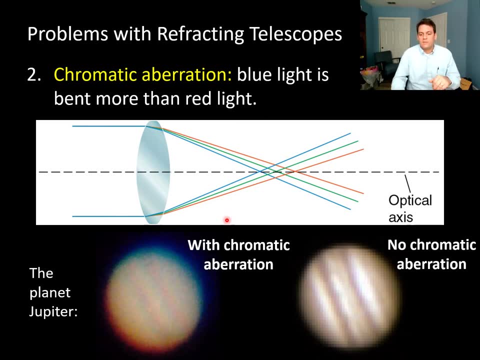 you know you have an aberrant color that you produce and so just to give you an example, looking at Jupiter, it's really a, it's a star effect here. I mean, you're used to the. I'm sure you've seen pictures of Jupiter before. these are not. 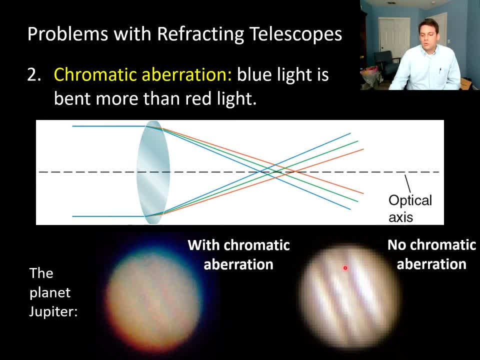 the highest resolution images that you've ever seen, and so you can see that images out there, certainly. but you can see on the right that looks like Jupiter. you can see the bands of clouds and certainly you probably recognize that as Jupiter, whereas here on the left, with chromatic aberration, it's, it's pretty. 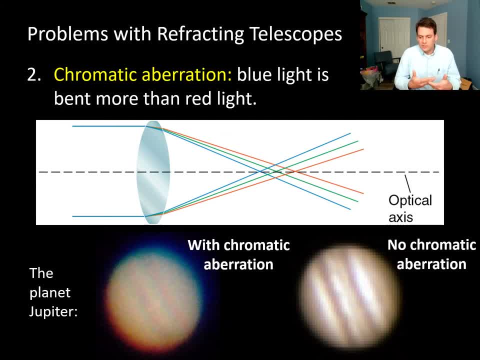 fuzzy right. I mean the colors are all kind of, you know, merged together. it's, you know, it's not that it's not kind of a cool picture still, but it's it's definitely not true to, to what's out there, and so this is a very serious limitation. you might have thought you. 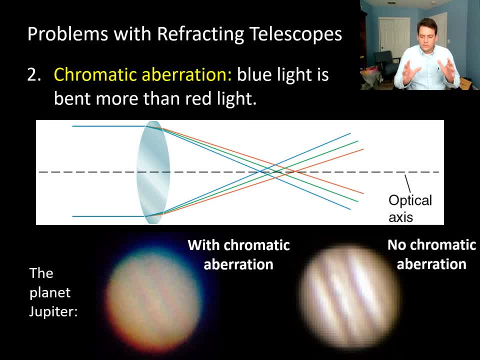 know, when it comes to just weight and length of things, you say, well, okay, it'll cost a lot of money, but we can find ways to engineer solutions to, to the practical problems of making very large refracting telescopes. but this is physics, just it comes from the physics of refraction and so there's no way to. 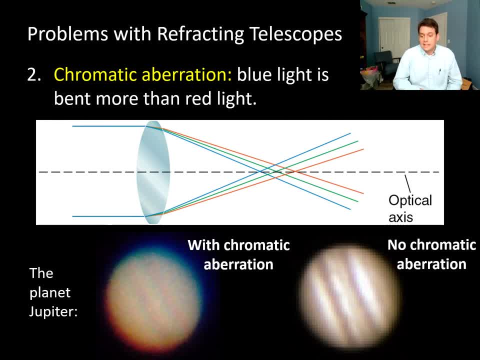 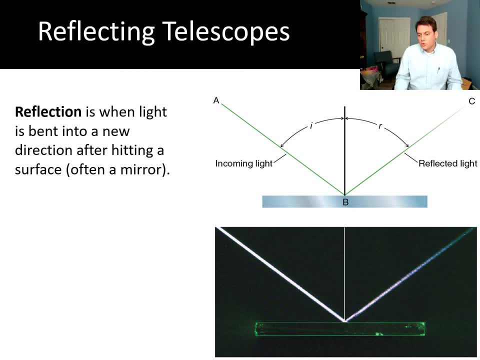 get around this, and it just gets worse and worse as the lenses get bigger. so the question now is: okay, what are we gonna do? we? basically, I just told you that we got from 1610 when Galileo first took, you know, his, his telescope and pointed up at the sky, and we made it into the 20th century with the Yerkes. 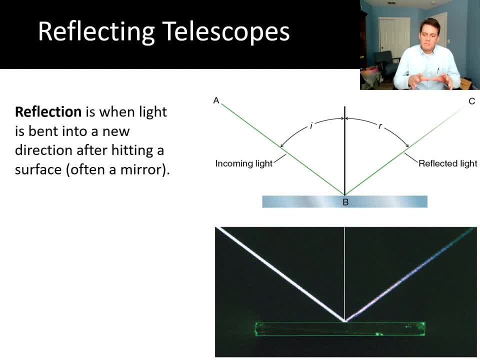 one-meter telescope. but you know, I just told us that basically we've hit a limit now what we can do in terms of refracting telescopes. so so does that mean that that we're just done, that we're gonna close up shop in the semester early? so unfortunately for you know, that's that's. 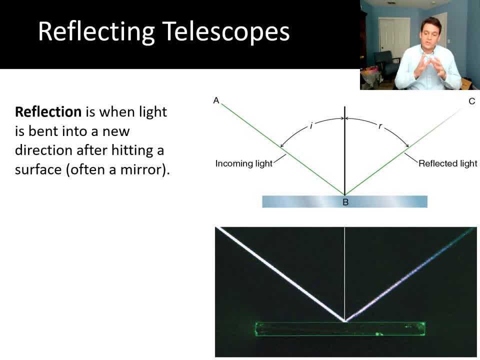 not the solution, that's. that's not the result, fortunately for astronomers. there is something else and, as you might have guessed from this slide, the something else is what's called a reflecting telescope. so, as you probably guessed, a reflecting telescope doesn't use refraction to bend rays. instead, it 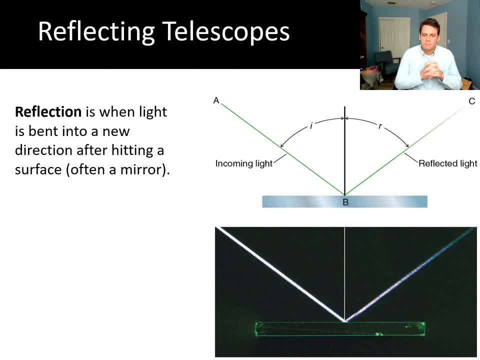 uses reflection from a mirror, and so the you know. whereas refraction used a lens to bend the rays, reflection is very straightforward. that's something you're you're familiar with. you have a ray of light come in, it hits a surface, it reflects, and what's called the angle of incidence, which is this angle here is 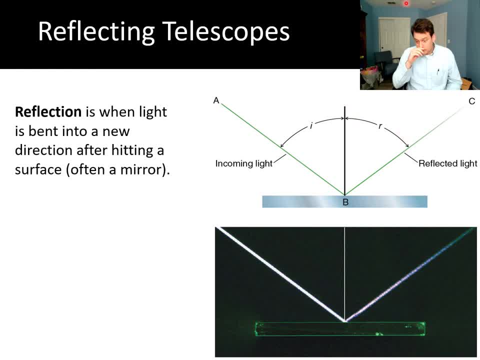 equal to the angle of reflection. somebody, somewhere, decided to give that statement, that sort of obvious statement, a fancy name and called it the law of reflection. so the angle of incidence is equal to the angle of reflection, and the great news about reflection is that the law of reflection is true for every way. 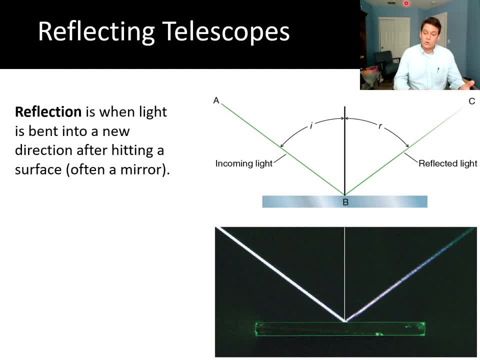 length equally right. so I told you that, when it comes to chromatic aberration, that exists because different light rays refract differently, different wavelengths refract differently. every wavelength reflects the same and it reflects at the same angle that it is incident at. so so, immediately, if we can find a way to, 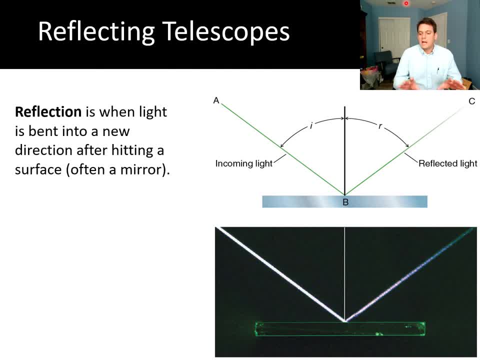 design a telescope using reflection. we know that chromatic aberration will not be an issue. so the question now is: well, how are we going to use reflection to to focus the rays? because, remember, focusing is is the is the job, that's the task at hand. when 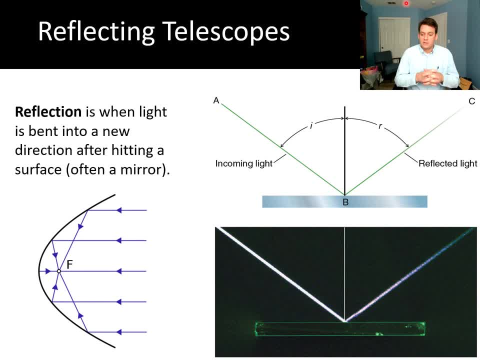 we're designing a telescope, we need to focus these parallel rays into a point, and it turns out that the way to do that, ideally, is with something called a parabolic mirror. and so, if you remember your algebra two days and your study of content sections, parabola is one of the 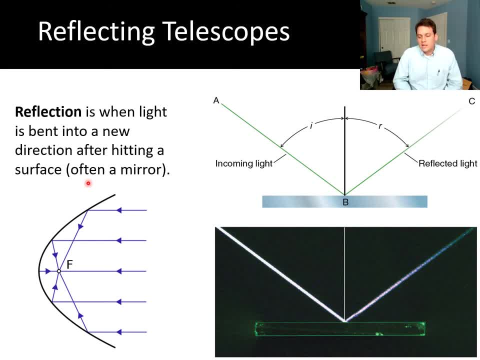 unit, and it turns out that- and you can prove this mathematically if you, if you like too- it turns out that a parabolic mirror is the correct shape to perfectly focus all of these rays down to a point, and so it's a little bit more complicated in the sense that you know we could draw. 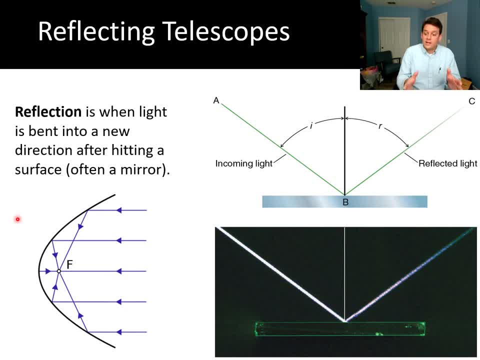 our schematics very easily using a refraction refraction mechanism and we'd set and we could see that fingerprint would be effected by reflection and we'd add repayment once that we draw the line in all directions. we drawitti KENCH, MATTIS. it's very easy. we just sometimes put it further than we supposed to put and those options are the same. so we couldização, you know, we could draw our schematics very easily using a refraction refraction mechanism and we can set and we could see it as this: 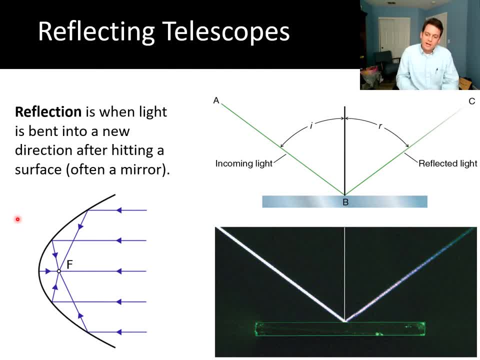 how these rays get focused down to a point and you put a screen there or you put a secondary, an eyepiece, you know lens and then, and then you can kind of stick your head down there. it's a little bit more complicated with refracting telescope, in the sense that you've reflected, or with a reflecting telescope. 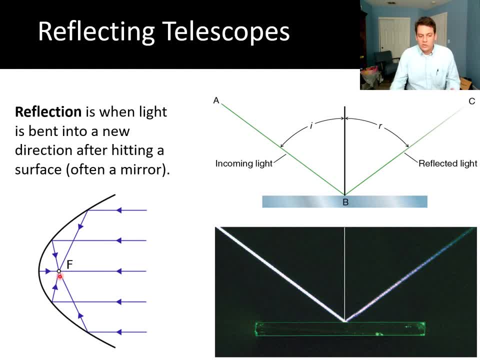 rather, you've reflected those rays back on to one another and so they do come to a focus, but that focus is kind of here in the middle of the system. but you know we've- people have spent enough time thinking about it that that this works quite well. and so, as it turns out- and this is almost guaranteed to come up on- 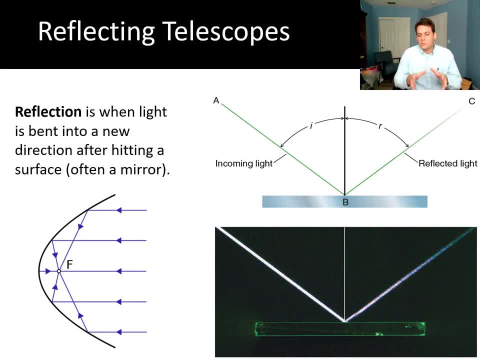 a test question at some point. reflecting telescopes are the more common sort of telescope now because they avoid chromatic aberration and, as it turns out, it's much easier to make a high quality mirror than it is a high-quality lens- grinding lens, lenses running glass down into. 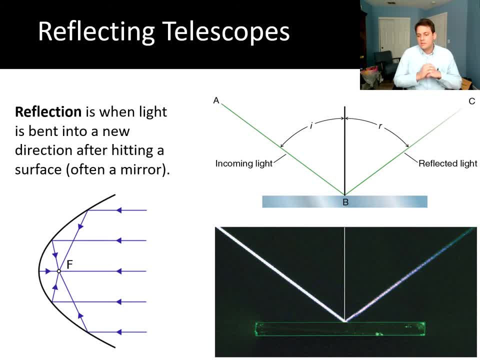 a size shapes is. we can do it, but it's not easy. and it's especially not easy when the lenses get larger mirrors. it's much easier and in fact mirrors don't have to be made of a single section. even they don't have to be, especially as they get. 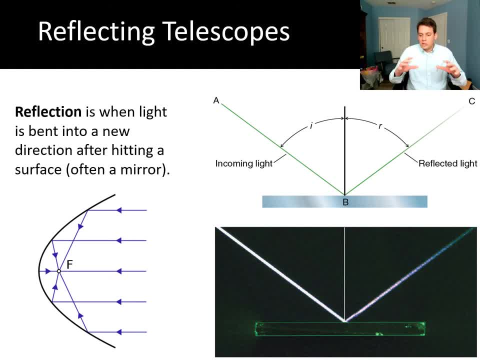 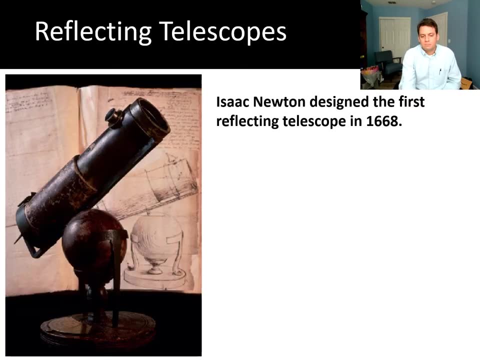 larger and larger. you can actually construct sort of a large mirror out of multiple pieces and and it's, and it's much lighter as well, because you don't have this huge piece of glass now, you just have some thin, you know piece, some silver surface which reflects light, so reflecting. 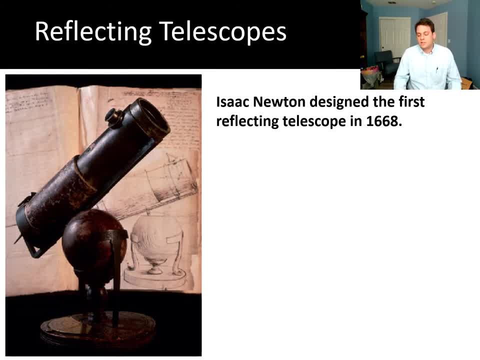 telescopes have been around for a long time. okay, so I kind of presented this initially by saying: you know, we started with reflect, with refraction telescopes, and then, and they, they were around for a long time and developed, and that's true, but reflecting telescopes did appear about 50 years, 50 or 60 years after the. 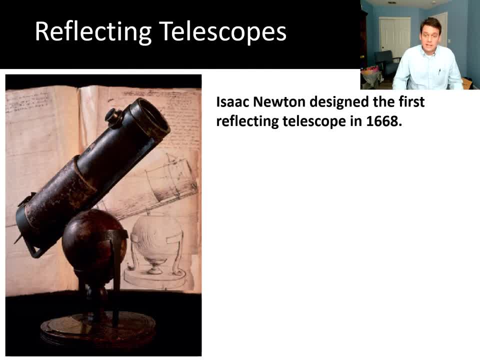 first, the first telescopes of any kind. right, and as it turns out, isaac newton is the first person known to have designed and built a reflecting telescope, and he did so in 1668.. and schematically it looks kind of like this. so again you start off with these. you know parallel rays coming from the distant star. 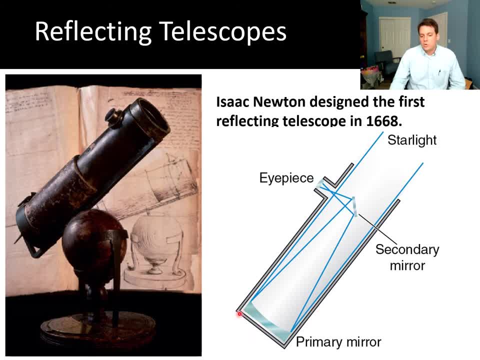 there was a primary mirror in the back of the telescope which was, you know, shaped carefully, and that reflected light back to a secondary mirror which then reflected it into an eyepiece, and that eyepiece would would still use a lens, right? because if you put a mirror here in the 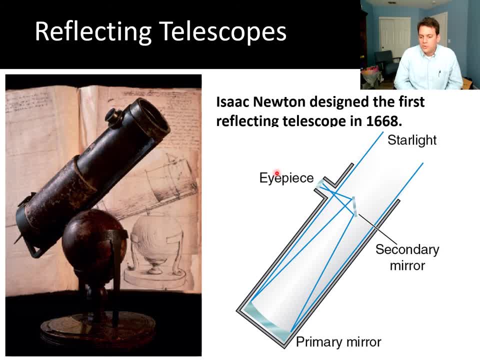 eyepiece, then you just reflect the light back into the telescope and you don't see anything, so that's not very useful. um, so you can't have an eyepiece lens here. um, but this is kind of the schematic of what newton designed in, uh, in the mid 17th century. 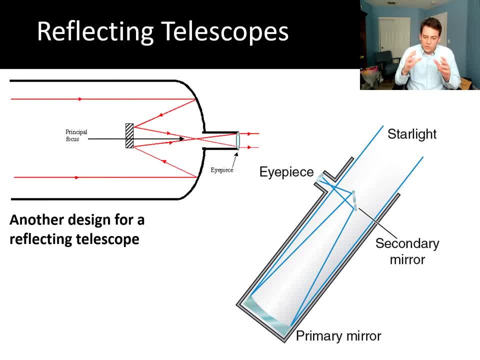 and there are other designs. so this is uh. this is something that if you were really excited about, experiment about the the detailed uh design aspects of telescopes. there's a whole lot of stuff out there so you can certainly get into that. we're not going to study that uh in a whole lot of. 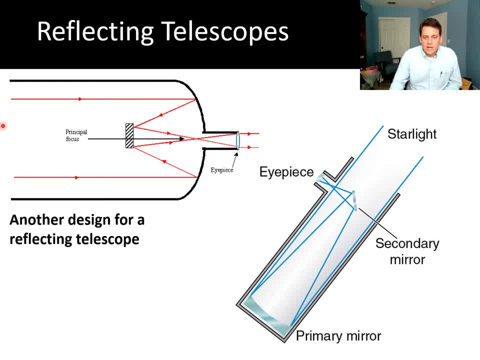 detail here, um, but the point is that there are, there are different options here. in this case you've got the. the primary mirror is kind of is again at the back of the tube, um, but then it reflects to a, a secondary mirror which is kind of in the middle, um, and then that reflects it back, you know, towards the eyepiece again. so 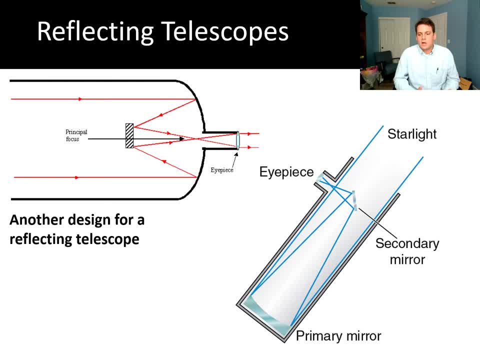 different designs, but it's the same basic features. you have a primary mirror, you have a secondary mirror, um and and again, you're using reflection not refraction, which means you avoid the problems with both chromatic aberration and the problems with these really, really heavy and unwieldy, very large refracting telescopes. 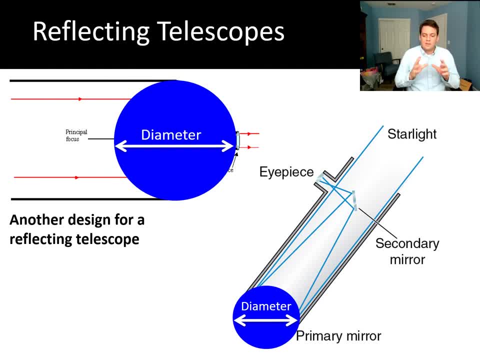 but just as with the refracting telescopes, the, the power of the telescope is going to be determined by the diameter of the aperture, um. so it's not, there's no lens here, right, it's a mirror, but but again, the, the size of that mirror, um is what's going to determine how much light. 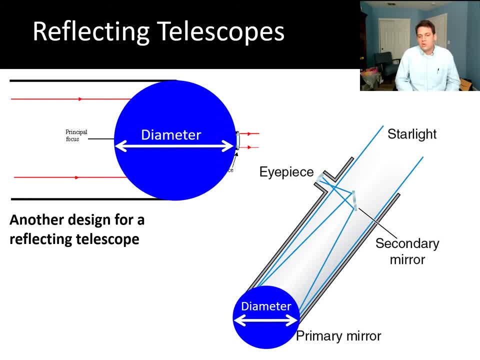 is being captured and and focused, and so the diameter of the of the mirror is going to be the sort of the most important piece in determining the power of the telescope. and, as i said, it's much easier to make a big mirror than to make a big lens. 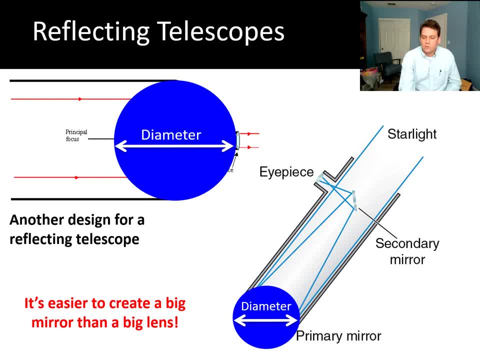 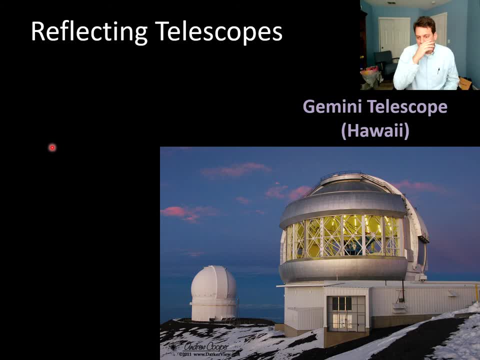 and so that's, that's one of the main selling points of these reflecting telescopes, and these things can get truly enormous. so here's one. you know, this may or may not look like a telescope to you, but it turns out it is um, it's the gemini telescope in hawaii. 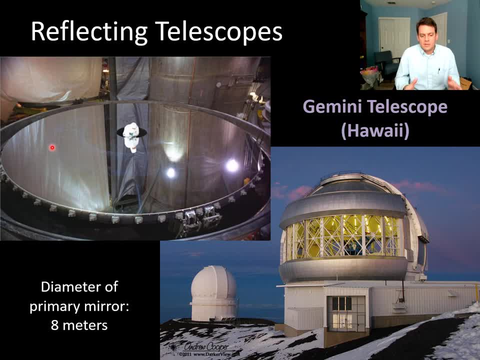 um, it's got a diameter. its primary mirror diameter is eight meters. okay, so i mentioned, you know, the yerkes uh telescope is the largest refracting telescope in the world. i had a diameter of one mirror, or one meter. um, and you basically can't get any bigger than that. well, we've got a primary mirror that is eight times that diameter. now, 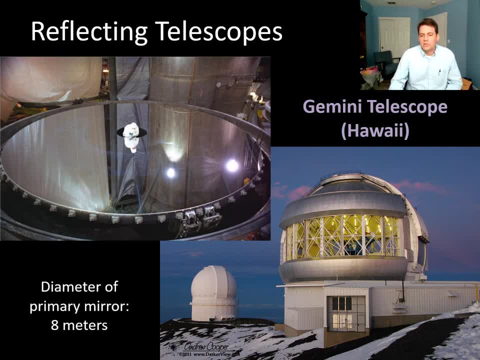 and, as i said, avoids the problems with chromatic aberration. so, um, it's, there's really no contest. you know, at this point, in terms of if you want to have a backyard telescope, you could go either way, it is more common to find a reflecting, to find reflecting telescopes. um the refracting. 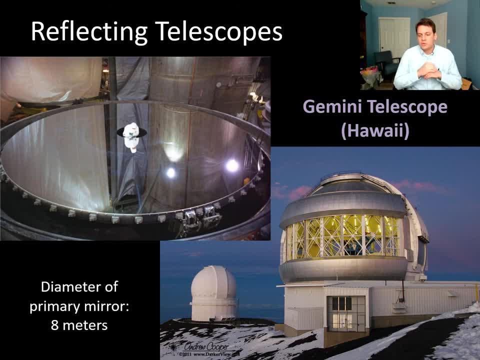 telescopes for backyard applications, but. but you can certainly find either and either would be would work. um, but you know, when you want to get to the cutting edge of of today's astronomy and really make new discoveries, there's just no way around it. it's got to be got to be a reflect. 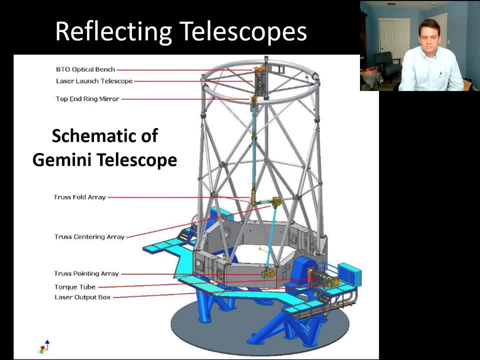 that would be a reflecting telescope. and here's a schematic of the gemini telescope. these things you know, they get when they get big, they get complicated, um and so lots of engineering and lots of details, and if you're interested you can certainly go go find out as much or or more than 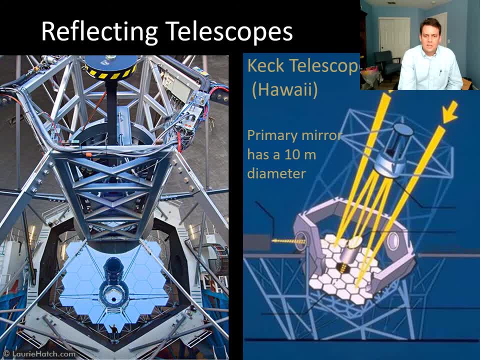 than you ever wanted to. another very famous uh telescope pushing the boundaries of astronomy today is the keck telescope, also in hawaii, um. it has a primary mirror that is 10 meters in diameter and, as you can see kind of from the schematic here, it is constructed in segments and so it's not just a single continuous piece. 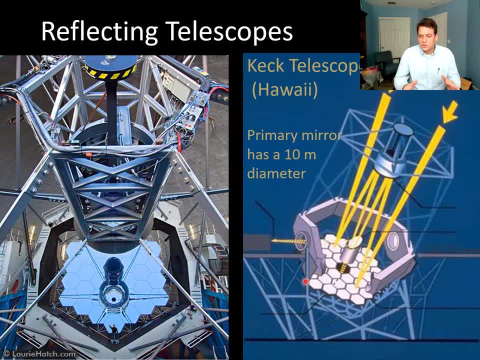 you know of mirror, because while those are easier to construct than than very large lenses, it still gets pretty difficult, you know, and unwieldy to construct. you know, a single continuous mirror that is, say, 10 meters in diameter, um, but it can be produced out of out of hexagonal segments, as it is here, and and work just as effectively. 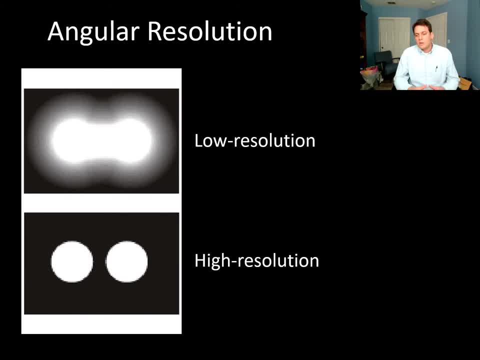 so let's talk a little bit about angular resolution. so i mentioned angular resolution is one of the most important characteristics of a telescope or your eye or any optical device, and certainly you hear about resolution all the time when it comes to, you know, tvs and computer monitors and so on as well, because a higher resolution gives you a better picture. 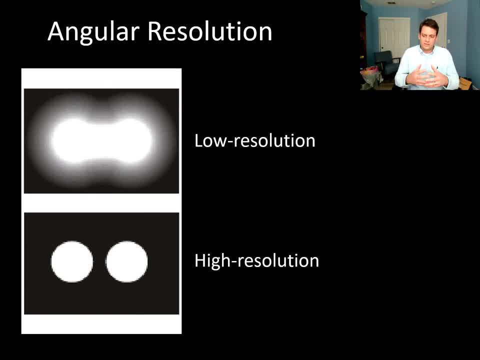 right, you can see more things more clearly, uh, the higher the resolution. and so this is this, and this is just a particular example where you can see if you have two, two things, two sources of light stars for us, but these could be headlights on a car or anything else, um, you know, at low resolution. 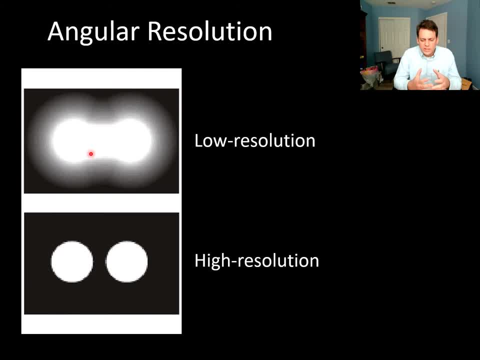 these things tend to merge together, and so you find yourself squinting and kind of trying to figure out. you know, is this, is this one thing, is it two things, five things? you know what's what's going on here, whereas with high resolution you have sharper edges. 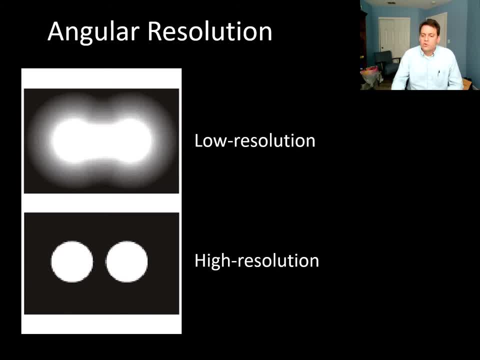 less fuzziness and you can clearly distinguish. okay, these are two different light sources. telescopes with larger apertures have better resolution. you collect more light, you focus it down, you get better resolution, and so that's why, in general, the push, you know, to discover more, to to learn more about the universe is, you know, almost inevitably a a chase to produce. 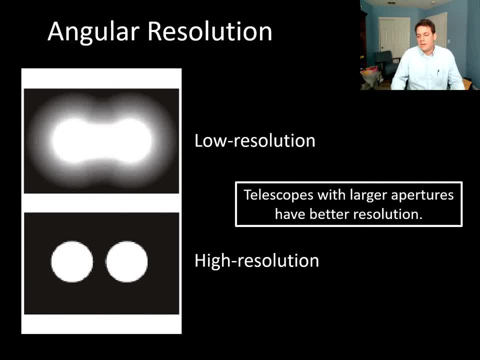 larger telescopes, telescopes with larger apertures, which means larger mirrors, in order to have better resolution. because if we, if we look out 14 billion years, 14 billion light years into the universe, but we don't have good angular resolution, then all we're going to see 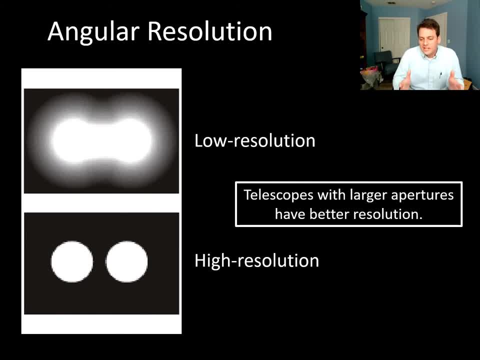 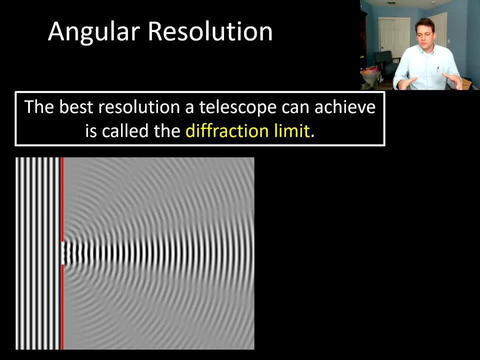 is a white, fuzzy, blur and you know we it's hard to learn a lot from that. so bigger apertures means better resolution, but unfortunately for us there is also a fundamental limit to to the universe and that is the diffraction limit. so the diffraction limit is the best resolution. 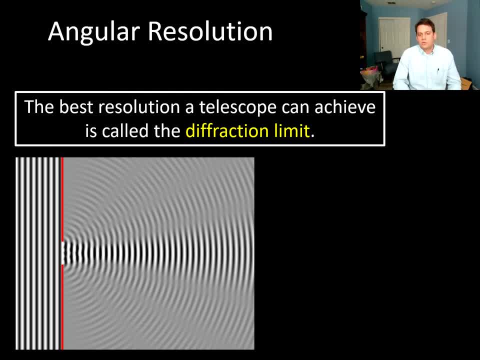 that a telescope can theoretically observe, and the reason that such a limit exists is kind of indicated by this: uh pinhole diffraction, uh sketch here, um, which shows something important, which is that when light, when waves of any kind, as a matter of fact. so this uh, this uh, 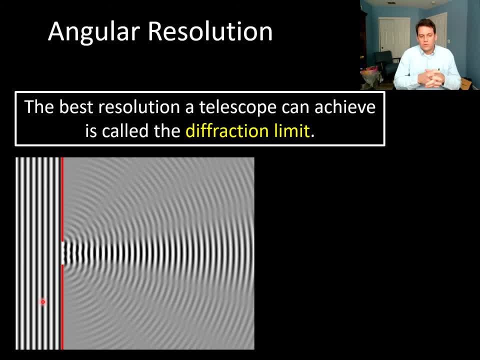 this is the diffraction limit, which is the best resolution that a telescope can theoretically observe. this could have been a water tank, for example, that did this experiment. but any time that waves pass through a, an opening, those waves diffract, and that means they, they end up bending. 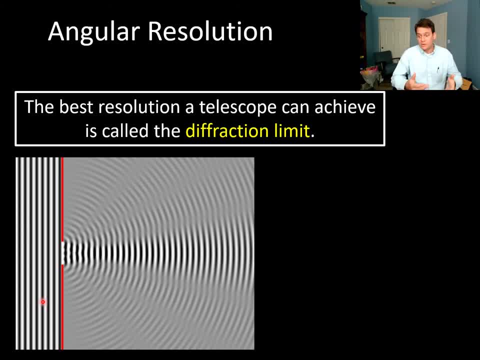 as they pass, either through a hole, in this case, or if they pass around an obstacle. so if you have, for example, if you have, water moving through a river and you put a rock in the middle, the the waves would diffract as they as it moves around there, and so um, because 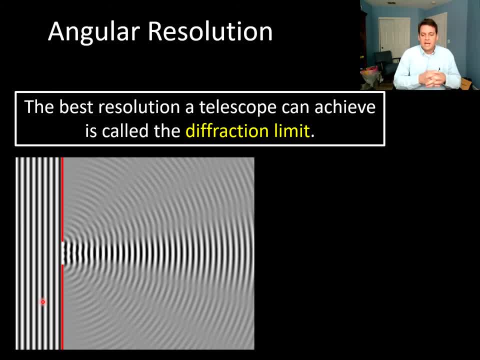 like because of the diffraction effect, as the light passes through into your telescope, as it moves into the aperture, it will be diffracted around the edges, and so, because of that, there actually is a fundamental limit called the diffraction limit, to the best angular resolution. 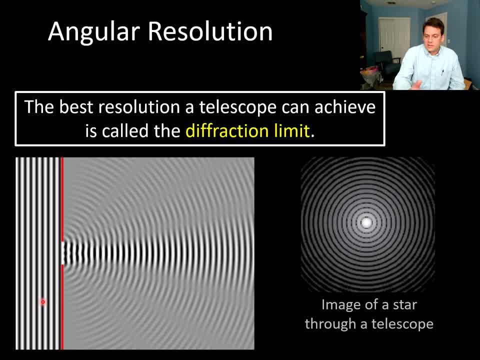 that you can get, and so, as a matter of fact, if you look at it with us with a circular aperture, if you look out at a star, for example, what you actually see, um, is something that looks like this: you have a central bright point, which is you know where that object is, but then you have these bright rings, concentric rings, that 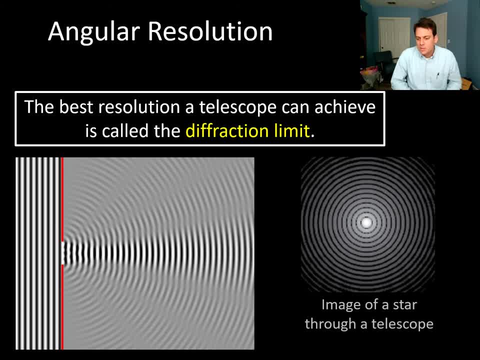 surround it um that are called diffraction maxima. um and again, if this were a physics class, we would go into some detail and study diffraction. it's uh, there's a lot, a lot of math you can do there and there's a a lot of things that you can learn um, but for our purposes, we don't like diffraction. 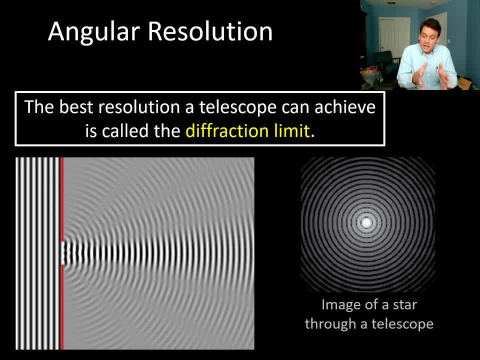 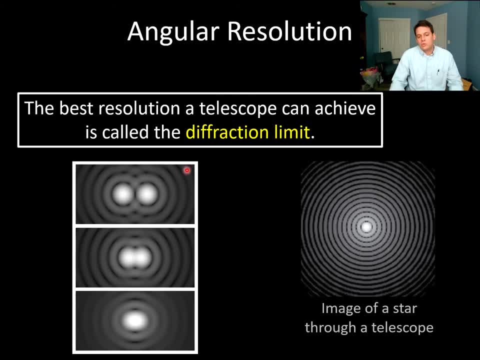 we go as far as where the light is. Jeremy, have you got the painting there? oh yeah, so of course, but we've all seen the top focal length. you have photo story about that. so color-based th force is exactly. that is obvious. there is a. there's no switching, but you can see that the component is so divisible. 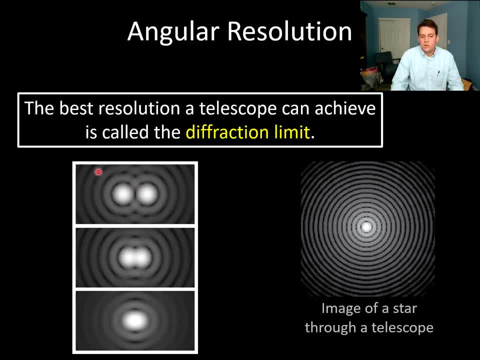 and so these are its successors. so, in terms of you know, blurring out what's being Näennie, this book subject value is to sort of sketch out your own and to send shots to the light sources, because if you're polar, Time law didn't start, it criticizes light, and so let me move on slightly. 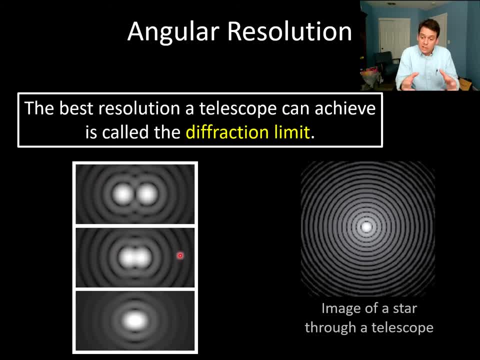 there are two light sources again on the other side is the 수 Law, because one of them, you can Пол them. But as they get closer, as these objects get closer, smaller you know angular displacement between the two, angular separation, these diffraction patterns start to merge, And so 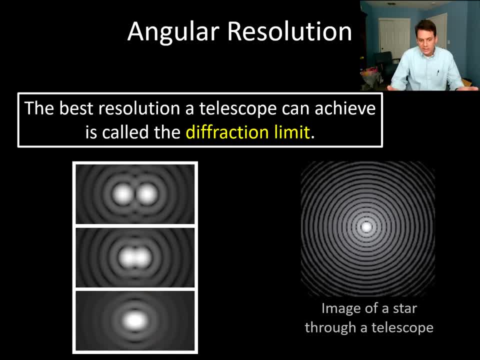 finally, you get down to this bottom picture and you look at that and some people would squint and say, yeah, I think I can see two different objects, but they're close. And other people would look at this and say, no, that's just one object, right? And so this is a good example of 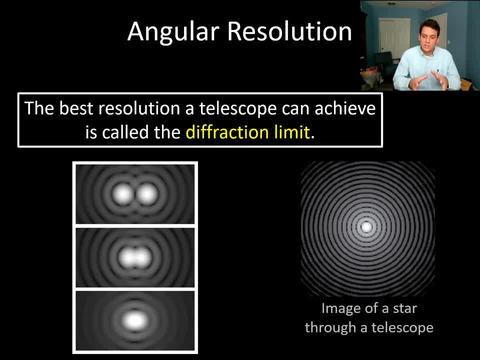 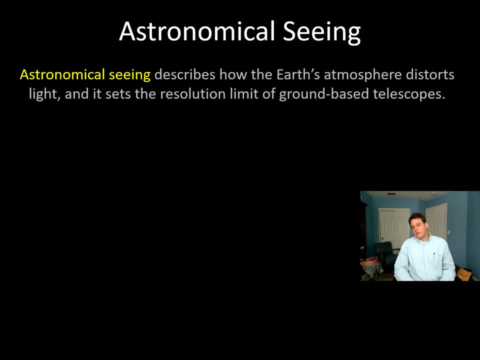 how the diffraction, how the diffraction limit really does prevent us from getting infinite resolution. So there's. there's another problem that can arise in the context of observations as well, whether you're using refracting or reflecting telescopes, And that's something. 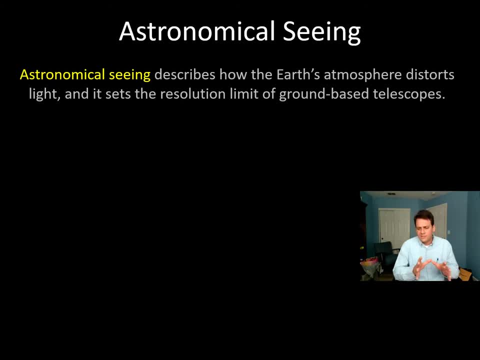 that is called astronomical seeing. Now I've I've made comments several times already that we're not very creative in our naming schemes. I kind of wish we'd been a little more creative. I wish we'd been a little more creative in our naming schemes. I wish we'd. 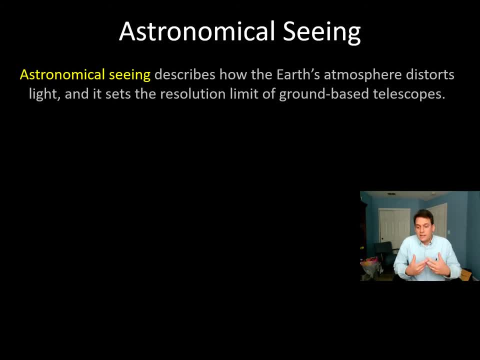 been a little more creative here because I have no idea what I mean. I do know what astronomical seeing is. I'm telling you what it is, but it doesn't convey a whole lot just by the term. but basically it's a not very technical sounding technical term for saying. 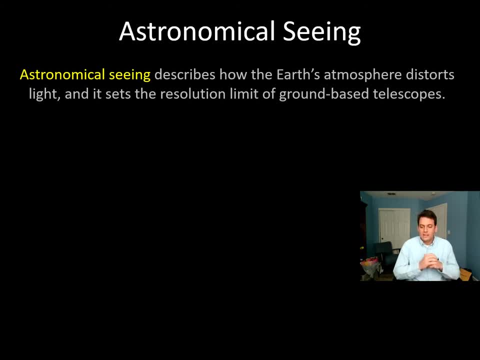 that the earth's atmosphere distorts what we view. And you know you may have already heard this, but you know, if not, I'll go on the record as saying: you know, stars don't actually twinkle right. Stars give off light at a pretty darn regular um. 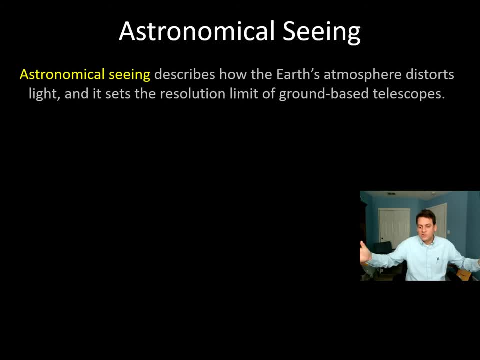 rate, um, over lots of years. you know they may vary some, but certainly when you're looking up at a star, it's not pulsing, Okay, Um, what's happening is that the atmosphere is in between you and the star, And so the star's light comes. who knows how many light years. 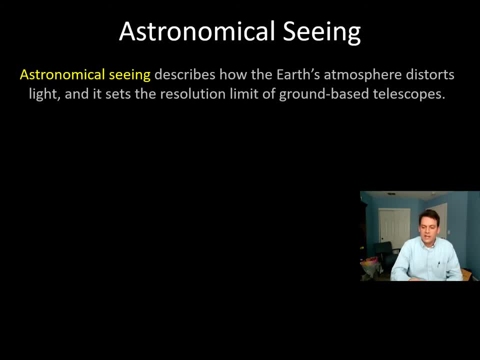 to earth, passing through the vacuum of space And then finally, just before it gets to your eyes, it passes through the earth's atmosphere and gets totally warped. Maybe not totally warped, but it gets warped by the atmosphere. Um, and, as it turns out, there's a lot of 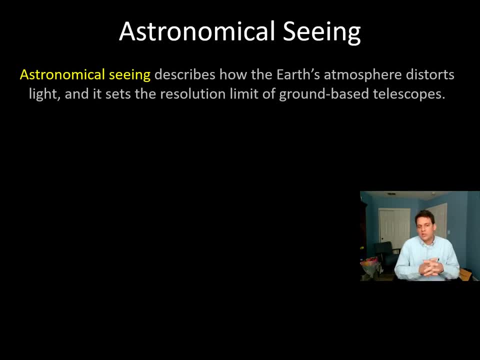 light in the atmosphere. So that effect is what's responsible for setting the resolution limit of ground-based telescopes. So you know, we've talked about chromatic aberration, We've talked about um, the diffraction limit, Um, but the the diffraction limit, while 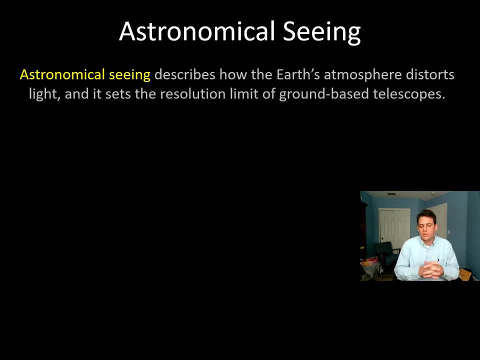 it does provide a theoretical limit for the best resolution that you could observe or that you could achieve for a given aperture and wavelength of light. um, you'll never get close to that. Okay, So the the thing that you know we're. 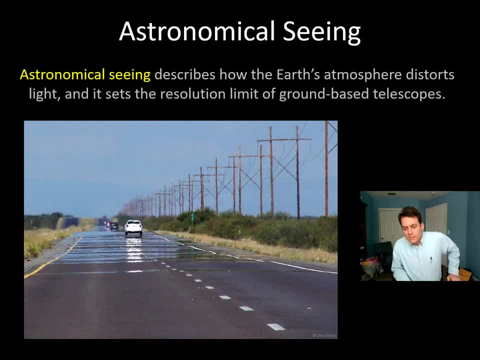 we've, we're used to, we're probably used to working with, with ground-based telescopes because of the, because of astronomical scene, because of the effect of the atmosphere, And you know, while this is not a telescopic image, um, one example of the atmosphere, uh, playing. 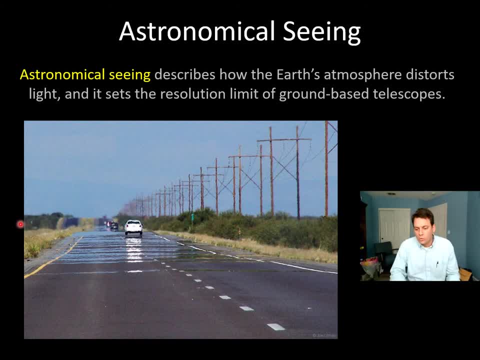 optical tricks on you is. And then you get up there and you realize, no, there's no water. And you think: is my mind playing tricks on me? Well, it could be that, yes, your mind is playing tricks on you, But it's also very often just physics here, where the heat of the road is such that the air next to the road is a little bit hotter than the air above it. 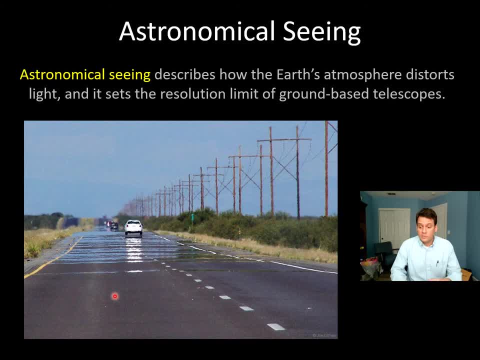 And so effectively. then, from an optics perspective, from the point of refraction, there are two different media, because light travels a little bit faster in the hotter air than it does in the cooler air, And so the result is that, just like light bends or can even reflect when it moves from one material into another, that can happen as light moves from cold air. 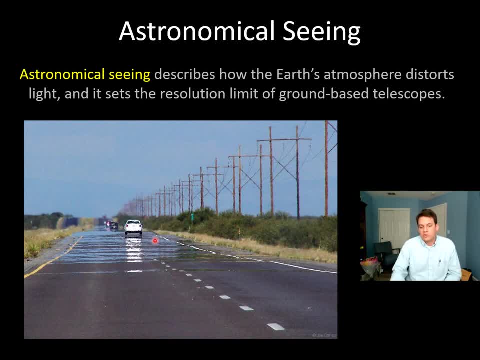 And so, in fact, when you look at this, it looks like you're seeing water. What you're actually seeing is the sky. Light is coming from the sky. It's not even making it to the ground, but is reflecting off of the hot air effectively and then coming up to you. 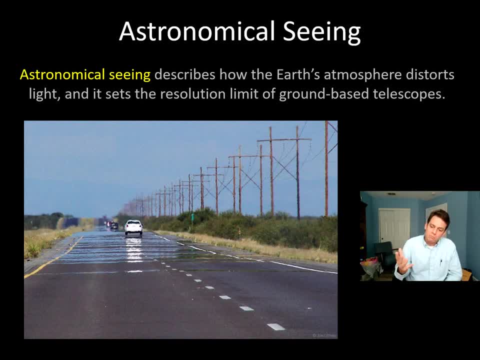 And so you're looking down and you think you're seeing something on the ground. Really, what you're seeing is the sky. So I remember when I first learned that, I thought that was pretty cool. And it's not. It's not directly applicable to you. know, we don't normally point our telescopes at the ground, so it's not something that we're going to do specifically here, but the physics is the same. 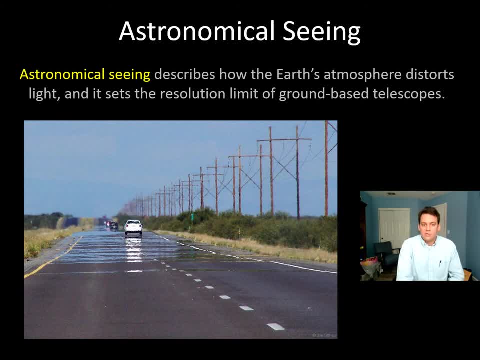 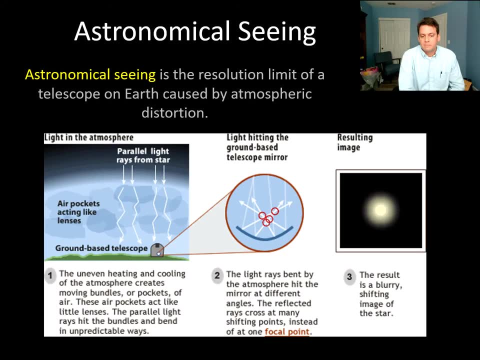 And it's sort of a very clear example of the fact that you're not seeing what you think you're seeing and the you know because of atmospheric effects. So how exactly does the atmosphere mess with our astronomical observations? It's easy to say it and I don't think any of you would probably argue with me, but what is actually happening? 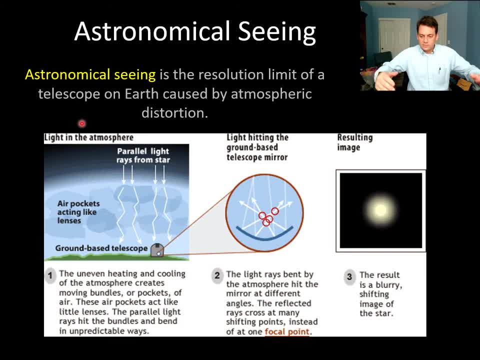 So these parallel rays come from stars out in the cosmos and again they travel who knows how many light years in straight lines, maybe occasionally passing through a cloud of hot or cool gas, you know out there, but mostly just passing through nothing. 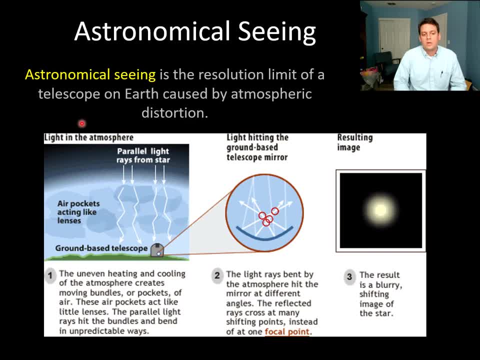 And then, finally, it hits the atmosphere just before it gets to us. So there's uneven heating in the atmosphere And cooling right. So there are pockets of atmosphere that are hot, there are pockets of atmosphere that are cold, and hot air rises and cold air falls, and so the atmosphere is always moving. 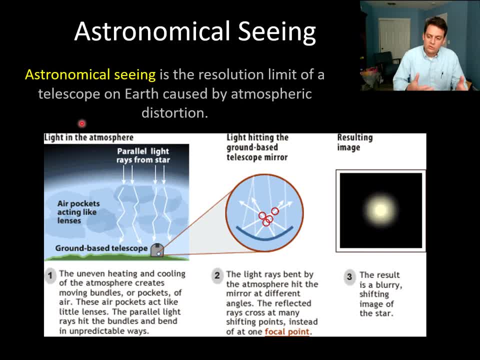 There are convection currents, sometimes storms, but there's always, even when it looks like it's clear, the atmosphere is always doing something. When that light enters the atmosphere, then it's going to hit these pockets And respond in. you know, I've said unpredictable ways here. 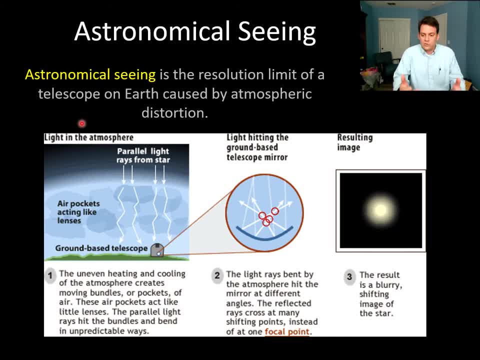 In principle it's predictable. We understand the physics. It's not like there's new physics here, But in practice it's going to look very random. okay, Because we can't, you know. you never know when a hot pocket of air is going to come through or a cold pocket of air. 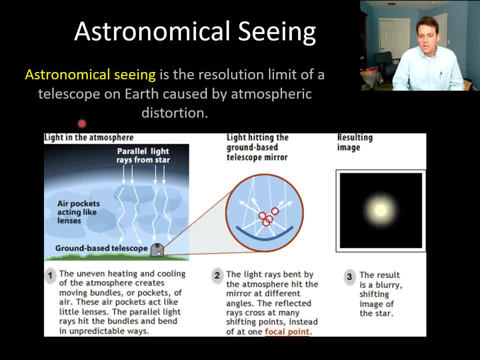 And so the result is that you've added randomness into these rays, So they were parallel, but now they're not quite parallel. They're a little bit off kilter, Because as they move through Hot air they get bent less than they would if they were moving through cold air. 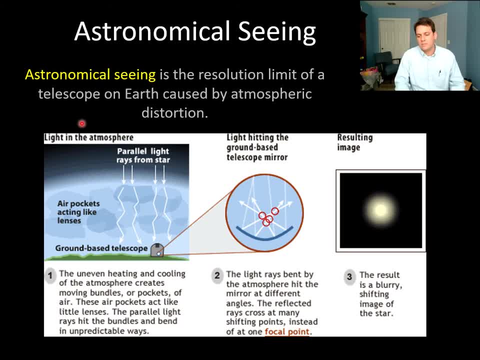 And so some rays are bent a little bit, and some rays are bent a little bit less, And the result is that when they finally hit your mirror or when they finally go through your lens, you know, in your telescope they're not actually parallel anymore. 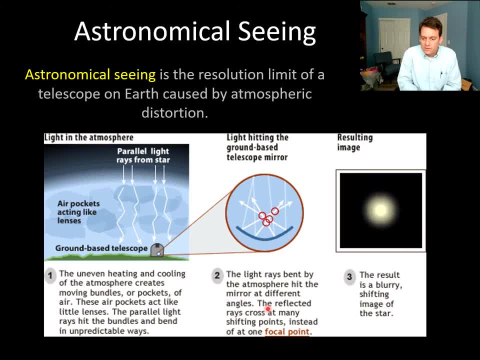 And so, instead of having a focal point, now, you don't. Okay, we're not a perfect one, right? Because the rays are still mostly parallel, But not completely, And so the result is they no longer focus perfectly to a point. 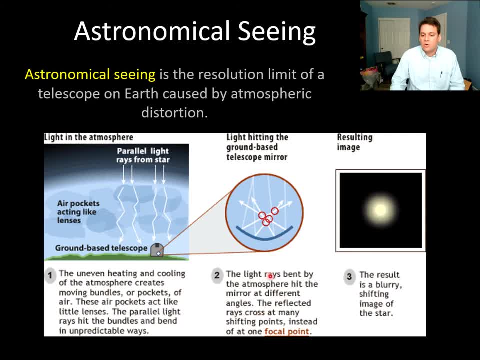 They're a little bit off, And so the result is that you get a fuzzy image, Okay, And you get one that changes over time. That's the twinkling again, right, Because as the air moves and so on, the rays get jiggled around. 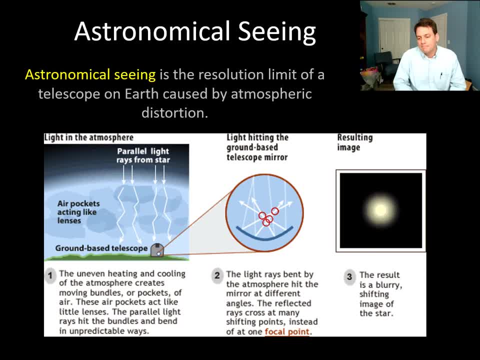 And so the focal points get jiggled around, And so the result is fuzziness And there's just no way around it. You know, As long as you're on Earth- right As long as you're on Earth, you know, safely ensconced in the atmosphere- it's great for you in terms of like ability to breathe and sort of regulate temperature and things like that, but there's no way around it. 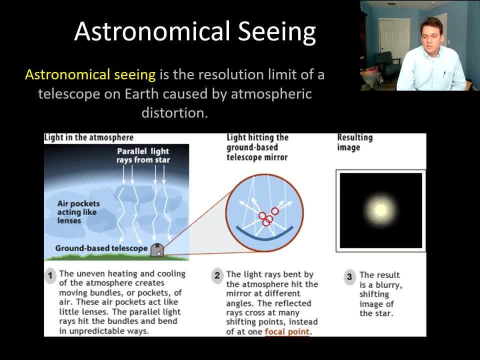 It's going to screw up your astronomy, And so that's just something that you either have to accept or try to get around, And there are a couple of ways to do that. The first, and maybe the most important one, is that you have to be able to get around. 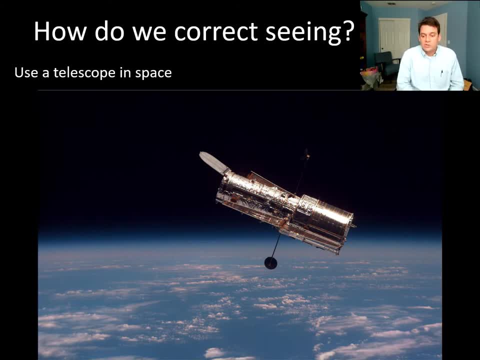 And there are a couple of ways to do that. The first, and maybe the most important one, is that you have to be able to get around, And there are a couple of ways to do that. The most well, yeah, the most obvious- is just get outside the atmosphere, okay. 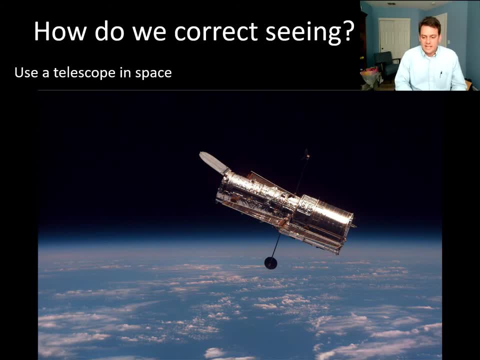 It's really expensive to do it. It's very difficult technologically and practically to put together something, as you know, as fancy as a high-tech telescope and then launch it into space and then, you know, put it out there in orbit and make sure that it doesn't, make sure it stays in orbit, doesn't crash back into, you know, to Earth. 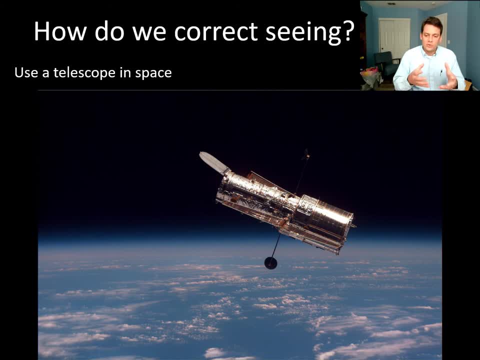 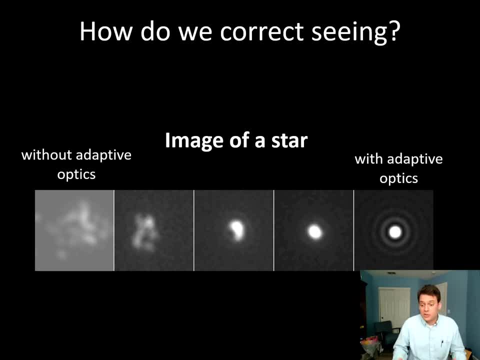 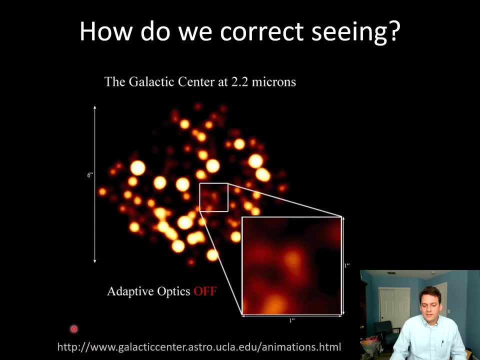 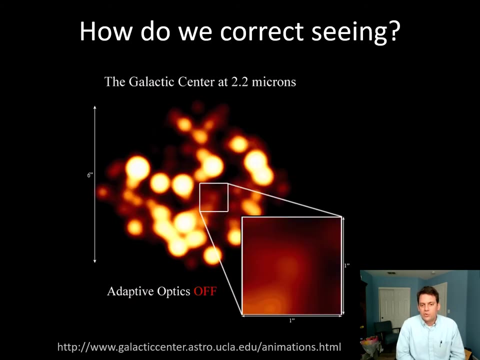 ground-based telescopes and still get extremely high-quality images. And there's a great animation here from UCLA that shows the application again of adaptive optics to the galactic center. So this is the center of the Milky Way. We're looking in there and trying. 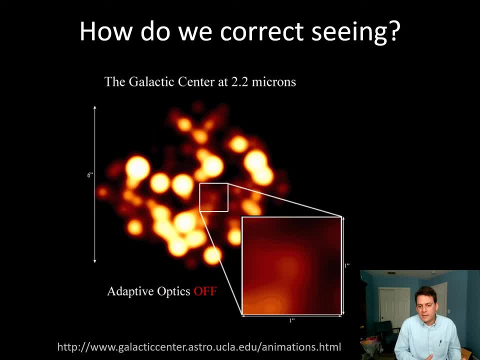 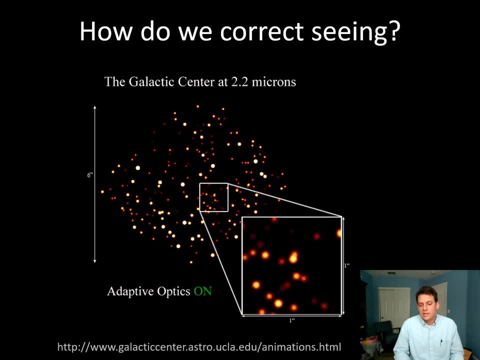 to get a sense of what's going on there. Without the adaptive optics you see some bright splotches- right, But that's really all. they are just splotches, Whereas as you sort of refine it with adaptive optics, you see very clearly individual bright spots emerge that are much 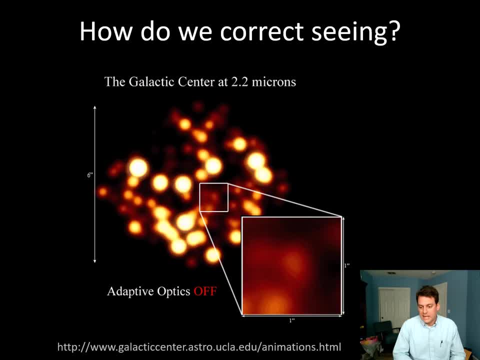 better resolved right. And so what began, what started off- just as like this red blur in space, in this zoom, in the zoom section- really becomes much, much more, much clearer, much more interesting, And so what we're trying to do here is we're trying to make sure that we're 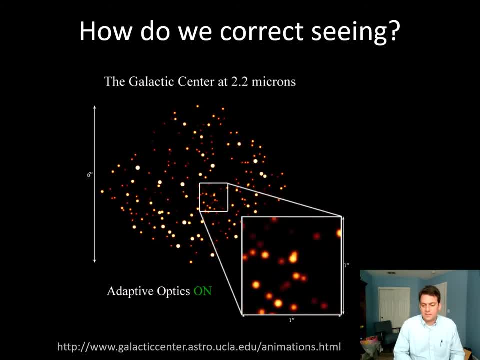 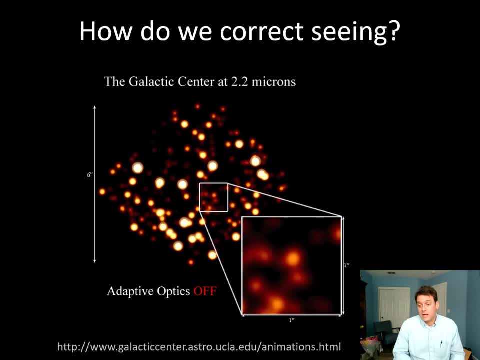 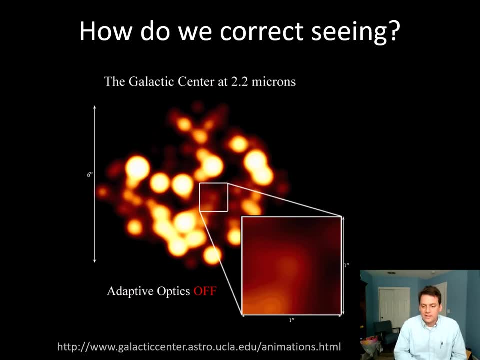 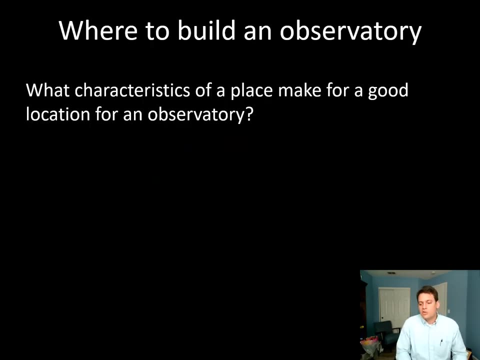 computer science does, but it's really phenomenal. So if anybody's interested, if anybody's not interested in that, you should be, but certainly I think that's a pretty exciting thing to probe further in if you're at all interested. Okay, so we've talked about telescopes. now We know. 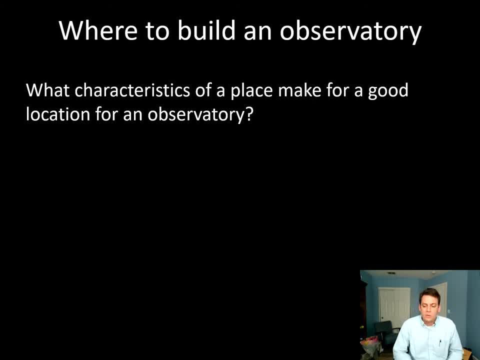 they're refracting telescopes and they're reflecting telescopes. We've talked about some of the limitations, both practical and fundamental. So now let's imagine we understand how to build a telescope. We've decided what kind of telescope we're going to build, Where. 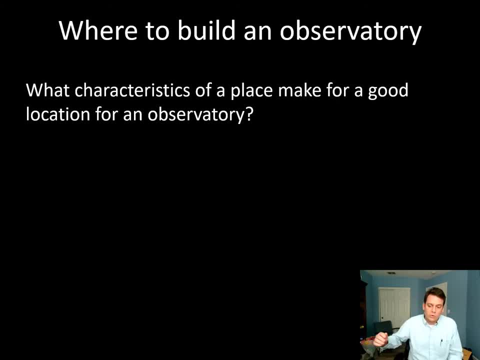 should we build it? Okay, So you know, do we just go build it? you know, knock down the neighbor's, you know houses, knock down the block of houses and, just you know, build it right there in my backyard, Or is there somewhere better? Well, there are a few characteristics. 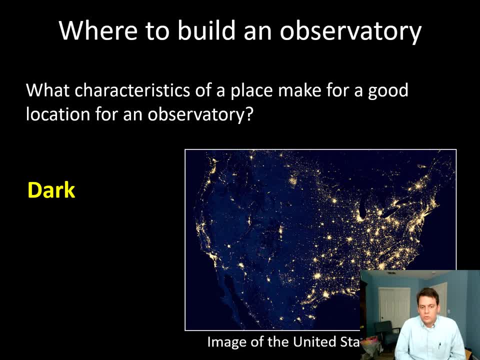 that are desirable for where you're going to build an observatory. And the first is kind of obvious, but let's go ahead and say it: It would be good if it were dark. Okay, It's, we're trying to see things that are pretty faint right in the sky, And so the 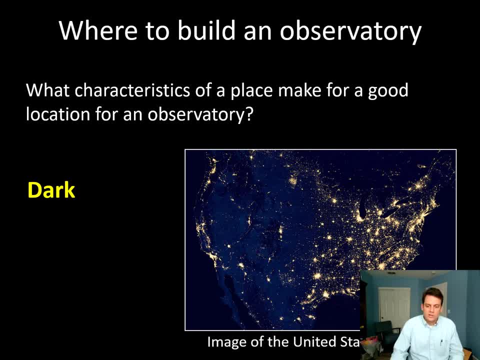 less ambient light you have, the better. Okay, So this is a nighttime image of the United States. You can see there's a lot of light in the US. The they're more dark in the United States. They're more dark in the United States. They're more dark in the United States. 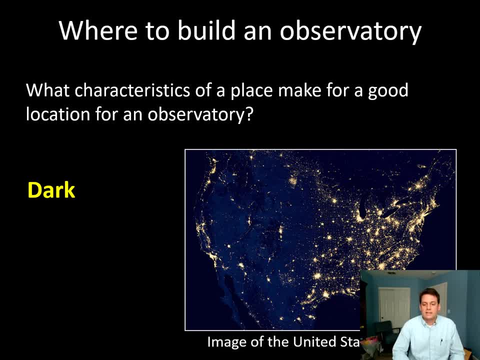 There are more dark areas out west than there are in the east, But but if you're going to build an observatory, you would like it to be dark, just so that the ambient light doesn't pollute your image. right, And if you've heard the term, light pollution is. 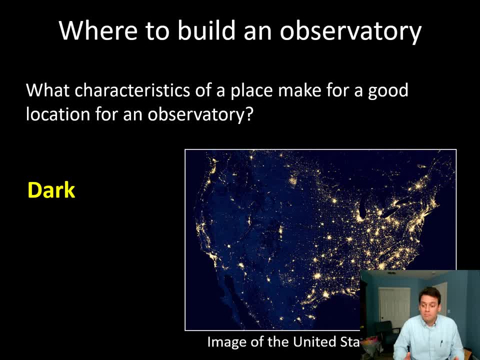 the term that's used with regard to astronomy anyway, and it is used more generally. You just you want a dark area so that you can see stuff better. The next thing that you would like is you would like it to be dry, And this is a very 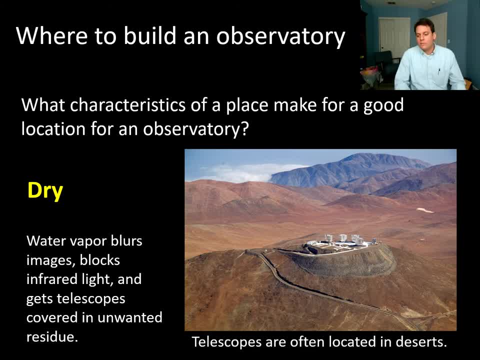 important thing, And this might be less obvious, But you know we've talked about astronomical seeing and the deleterious impact of the atmosphere on our observations, But it turns out that water vapor is particularly insidious when it comes to astronomical observations. So 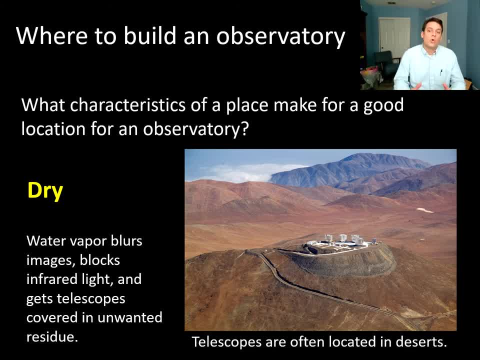 the more water vapor there is in the sky, the worse your image is going to be. And so- and there are a couple of reasons for that- It blurs the images, as we've discussed. It blocks infrared light. It blocks infrared light, which is a problem for infrared telescopes, You know again. 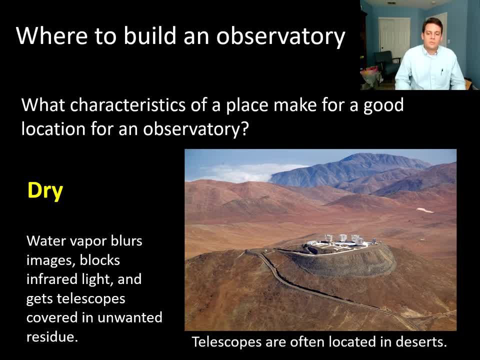 we tend to focus and tend to think about visible light telescopes, But a lot of the biggest and most powerful telescopes that are used now look at wavelengths outside of the visible range, And so infrared light can be blocked by water vapor. So that's not good, And if 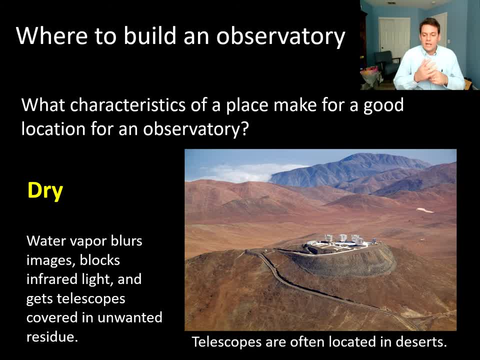 you have. if you've got moisture in the air, then when you're looking at the sky you're going to wake up in the morning. it will likely have gotten cool enough that it will condense, and then you'll get condensation on your instruments. Okay, And that's definitely. 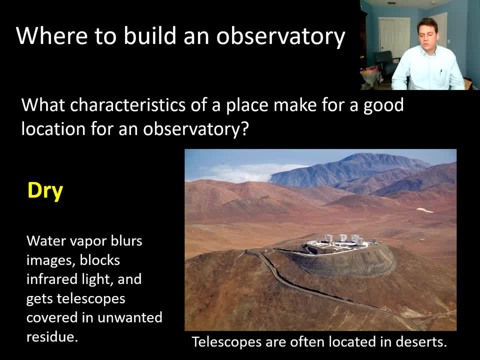 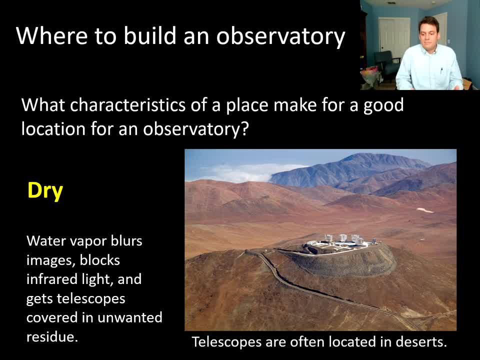 we want it to be dark. So if we're going to build an observatory, we want it to be dark. So if we're going to build an observatory, we want it to be dark So away from people, and we want it to be dry, so that we don't have these myriad of problems introduced by 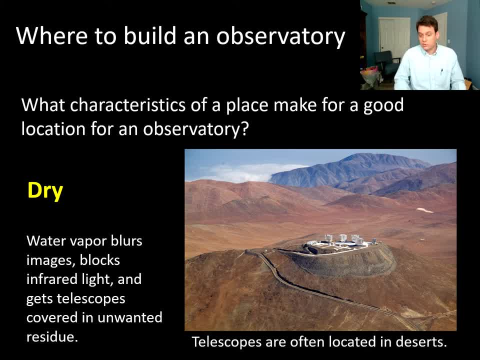 water, And so, as a result, telescopes are often located in deserts. Okay, So those are two characteristics When you're going to build your observatory. those are two characteristics that you want, And a third characteristic is that it would be good if this were high. 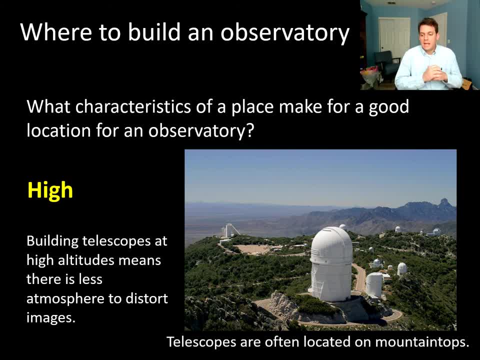 at high elevation. Okay, And that's again just a practical matter here, But the higher you are, the higher you're going to get, And so if you're going to build an observatory, the less atmosphere you have to see through, As you know, the higher you get in elevation. 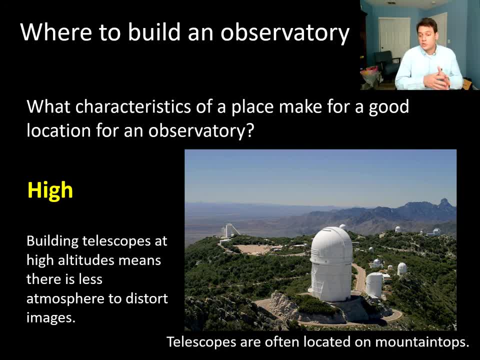 the lower the density of the atmosphere is, And this is noticeable even if you just climb a mountain right, Or if you go to Denver, the mild, high city, the atmospheric density drops, And so the less air that you're looking through, the less distortion that you're going. 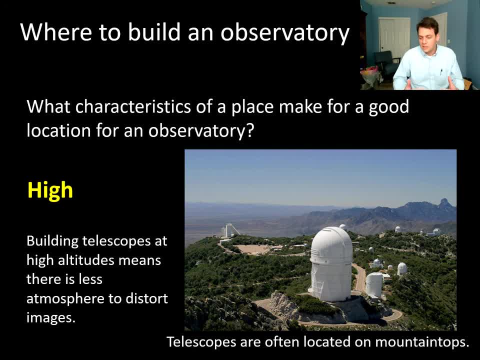 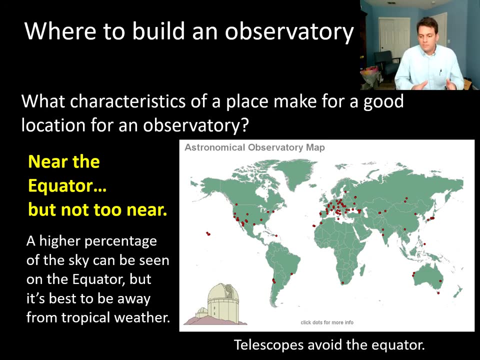 to have to either just accept or fix with adaptive optics and so on. So you'd like your location to be high, you'd like it to be dry and you'd like it to be dark, And finally, you'd like it to be near the equator, but not too near. Okay, And the reason for that? 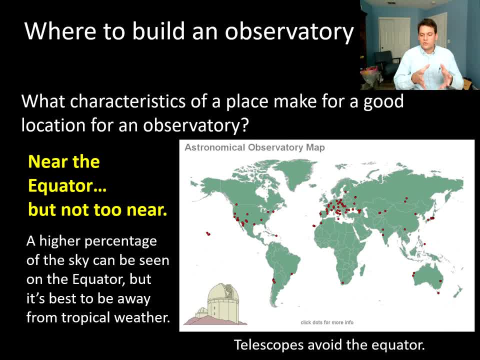 is that in the Northern Hemisphere you see certain stars at night and in the Southern Hemisphere you see different stars. If you're near the equator, you see more of the sky. You can see both Northern Hemisphere and Southern Hemisphere stars. 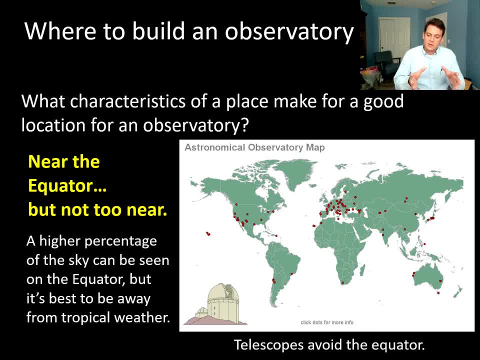 But, as you probably are aware, the closer you get to the equator, the more humid it tends to get as well, And so, and we just said that we would really like our ideal observatory to be located somewhere that's dry, And so you're trading things off here because you 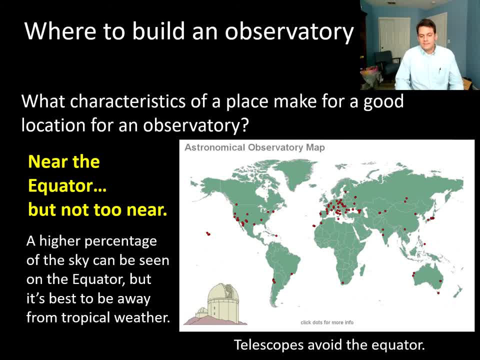 don't want all the moisture, you don't want the tropical weather, you know. you don't want rain, you don't want clouds. right, That's another. I didn't mention clouds before, but certainly if you're somewhere where it's wet enough, you're going to get clouds and then 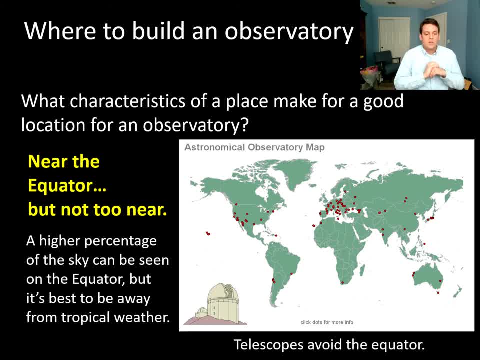 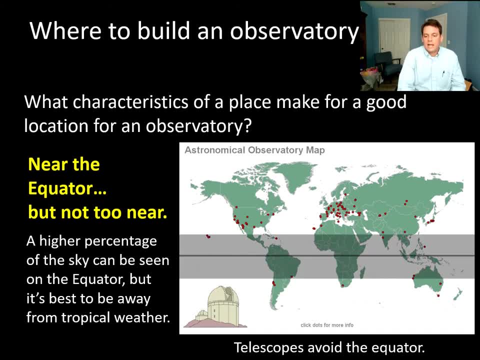 that's a total disaster. right for observing. So that's why you would like to be near the equator, but not too near, Okay, And so the gray region here are the tropics between the Tropic of Cancer and the Tropic of Capricorn. We tend to stay outside of those, so these 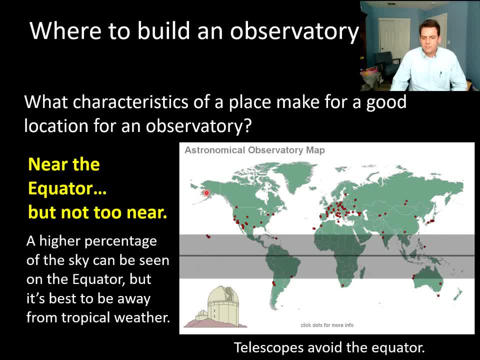 red dots are just just represent particular observatories around the world, And so you can see there are more in the United States and Europe than elsewhere. There are a few scattered around the world, though, And most of them are outside the tropics, You can see. 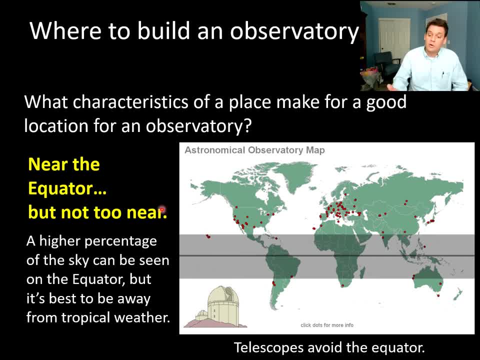 there are a few dots here in Hawaii. Those are up on very high elevations in the mountains, actually up above the clouds in most cases, And so if you have that situation, then you're okay, right, Because you say, well, we're in the tropics, but we're so high in elevation. 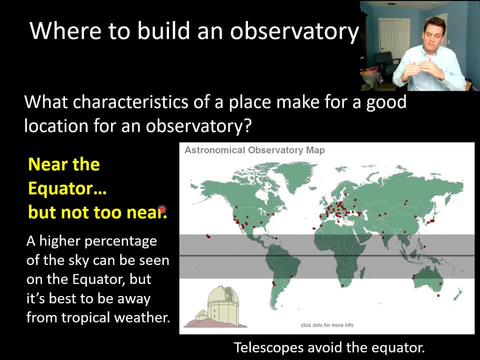 that effectively you've stepped out of the tropics now vertically rather than horizontally. But you see, there are quite a few locations kind of just outside the tropics, here in South America and then again in North Africa. Obviously you know these. as I mentioned, these are: 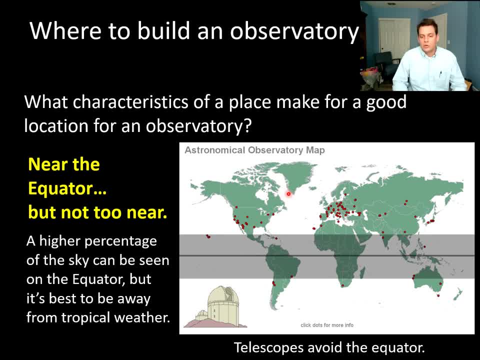 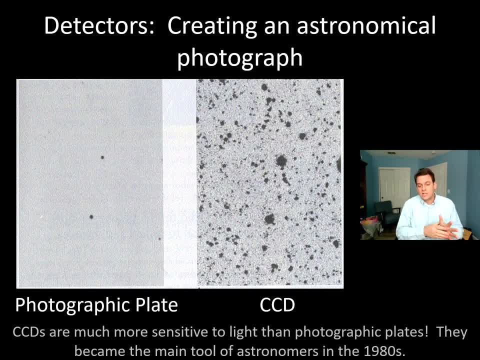 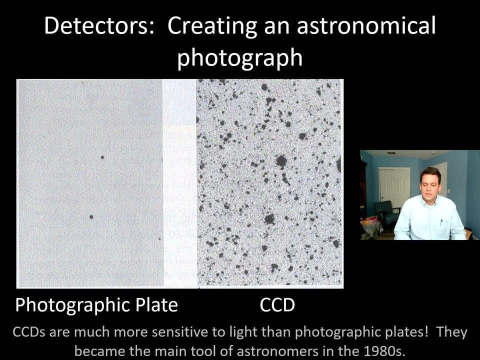 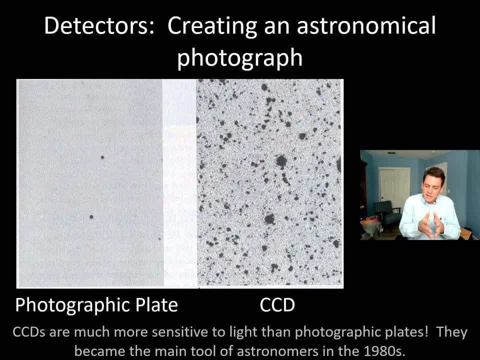 plates, The photographic plates, you know they rely on this chemical reaction. You have to have enough of those reactions occur to make a dark enough spot that you can, that you can clearly see it. um, And each cell is either activated or not. 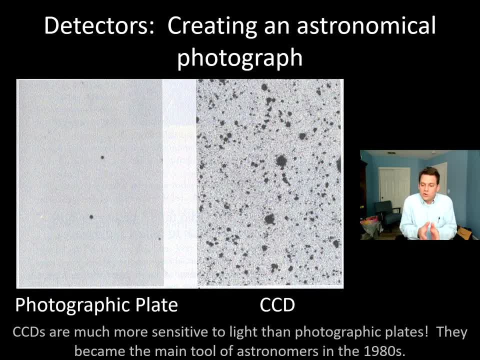 It's either, you know, light or dark, And we can put a whole lot of those onto a single CCD, And so that's what allows us to get such high resolution. So people do spend careers, you know, learning and applying the details of that technology. 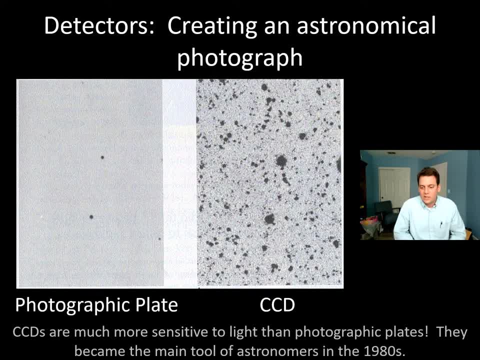 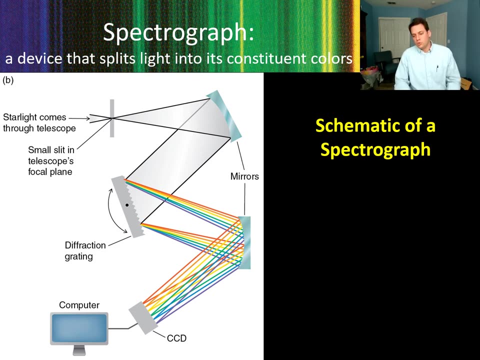 We're not going to do that. We just need to recognize and appreciate the fact that the development of the charge coupled device really did revolutionize our ability to get high quality, very high definition images. So there's another tool that you know. we spent most of the time today talking about telescopes. 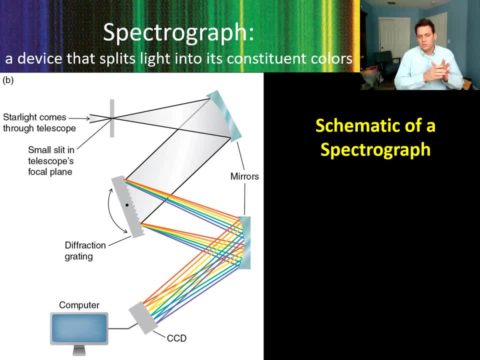 But there's another tool that we're going to refer to periodically, And particularly over the next several lectures, where we will move- We're going to move on after today- into analyzing starlight, And one very important tool in that context is called a spectrograph. 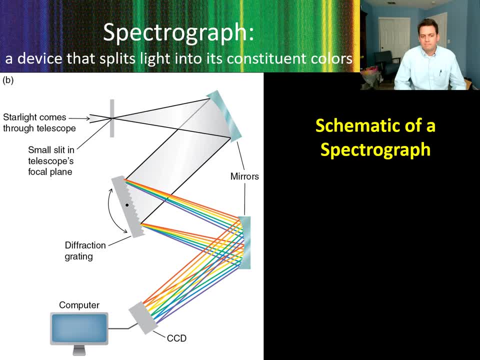 And it's a device that just splits light into its components. Okay, so white light is the combination of all colors, Right, all different wavelengths, But it turns out that we're going to be able to get a huge amount of information out of the light by splitting it up into its components. 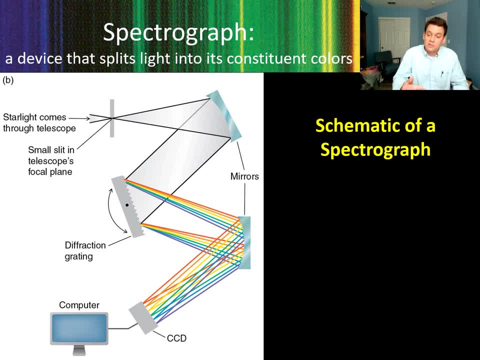 And seeing, how much of this wavelength do we have? How much of that wavelength do we have? Are there any wavelengths that are missing, for example, You know, if you think back to absorption line spectra. So basically, the way a spectrograph works is that light comes in through a small slit in the telescope's focal plane. 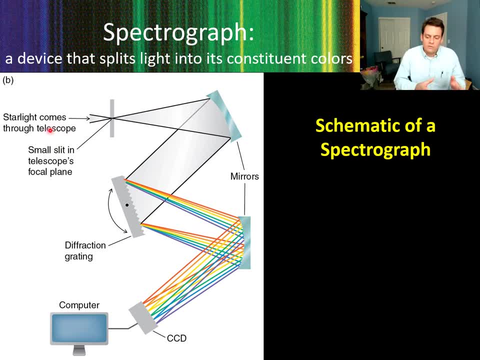 So again, you know whether you're using a refracting or reflecting telescope. light is focused to a focal plane. You then use mirrors to reflect. use a mirror to reflect it onto something called a diffraction gradient. Okay, And there are a couple of different ways of making diffraction gradients. 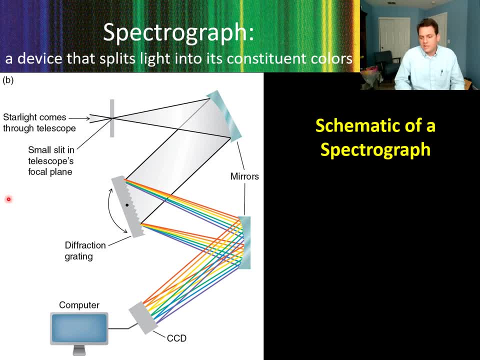 And we won't go into the details there. but the point is that it's something that splits light up into its colors. So you know, a prism does that using refraction Turns out. you can split them up using diffraction as well. 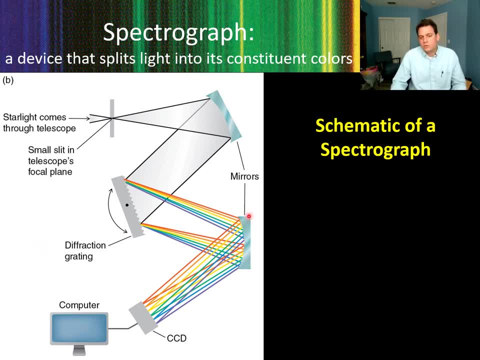 And that's what a diffraction gradient does. And then you use another mirror to reflect that, the diffracted light Now. so you've separated out the colors, the different wavelengths, You capture that with a CCD And you use some. 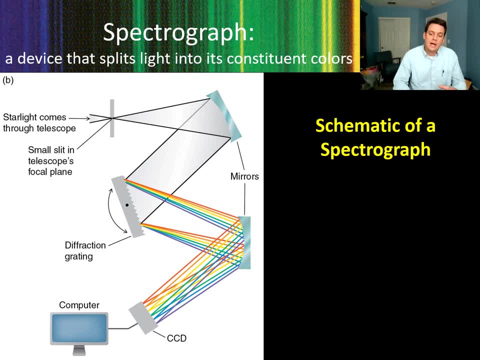 Fancy computer software And you can analyze exactly how much of this wavelength, how much of each wavelength, do you have? And you know, going forward in the next couple of weeks, we'll talk in a lot of detail about how we can use that information to figure out what the heck this stuff is that we're looking at. 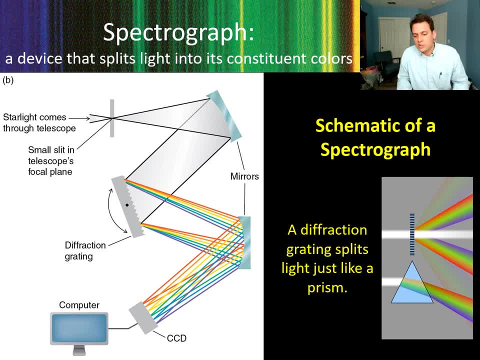 So, as I said, the diffraction rating splits light. Maybe I shouldn't say just like a prism, It splits it. They both split it, but they use different, different techniques. Right, Diffraction is The bending of light when it passes through a slit or or past a an obstacle, whereas refraction is the bending of light as it passes from one medium into another. 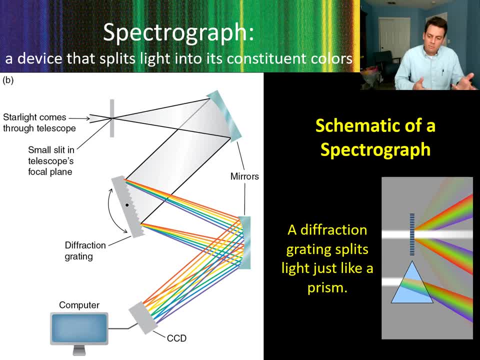 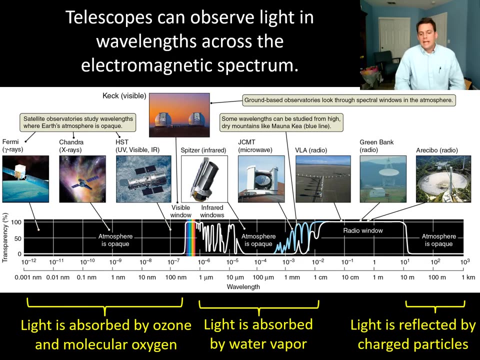 So both achieve the same results in terms of separating out light. Sometimes diffraction is more easily applied, Sometimes refraction is more easily applied, Just depends upon the application. But a spectrograph here uses a diffraction Really And, as I mentioned telescopes, we tend to focus on the visible range when we're in a visible spectrum, when we're thinking about them and certainly when we're visualizing them, because that's what we can visualize. 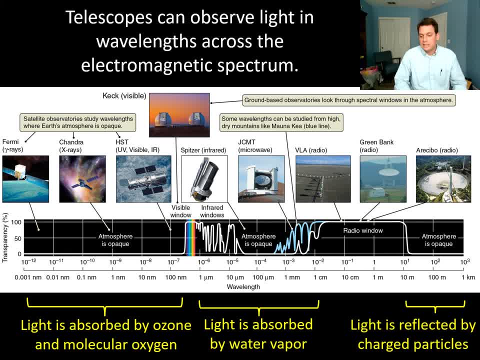 But after the discovery that, you know, visible light is just a very small sliver of the electromagnetic spectrum, happens to be the sliver that that humans eyes are attuned to. So it didn't take scientists long to realize: well, we might not be able to see these other wavelengths, but if we can detect them we might be able to get a lot of information. 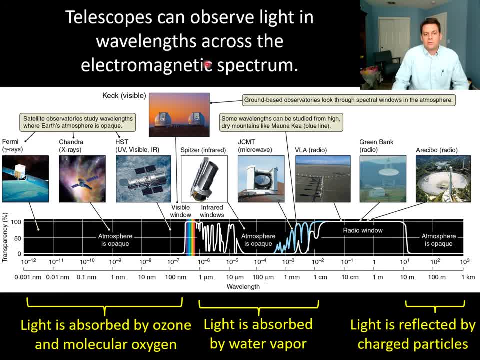 And it turns out that that's true, And so I'm certainly not going to read all of the slides to you, but I hope that it will convey to you the the fact that astronomers do actively now use essentially the entire electromagnetic spectrum. And so we've got, for example, on one end of the spectrum we've got the Fermi telescopes, which looks at gamma rays, which is the highest energy. 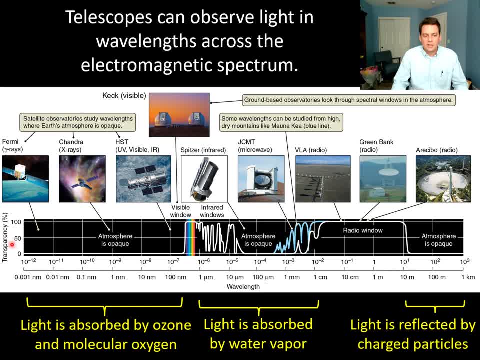 It's the highest energy portion of the electromagnetic spectrum They are, and so a Fermi telescope is outside the atmosphere. It's in orbit because those gamma rays don't survive the atmosphere. On the other end, we've got a lot of radio telescopes around the world, which are what they sound like. 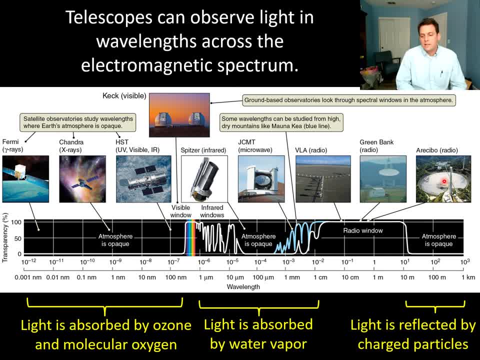 Instead of using visible, instead of detecting visible light, they focus on radio waves, And then we've got everything in between. One thing that's interesting and worth noting is that if you look at the transparency of the atmosphere here, as a function of the wavelength, it varies a lot. 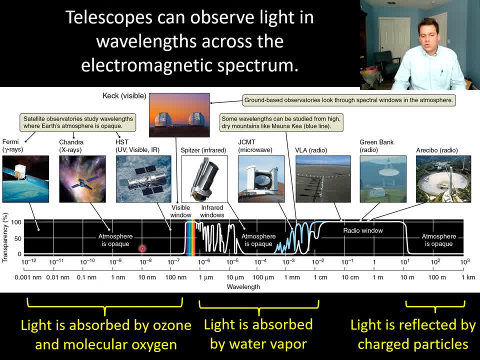 So the atmosphere is opaque to these very short wavelength electromagnetic waves. So this light is absorbed by ozone and molecular oxygen, of which, fortunately, we have quite a bit. Not the ozone, We do have some ozone. We're fortunate to have plenty of molecular oxygen in the atmosphere. 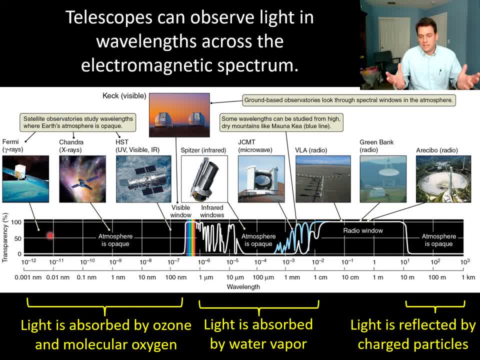 So that oxygen, just it takes care, it knocks out all of these, you know the X-rays, the UV and the gamma rays. Visible light gets through the atmosphere, right, That's why it's visible. If it didn't, then it wouldn't be. 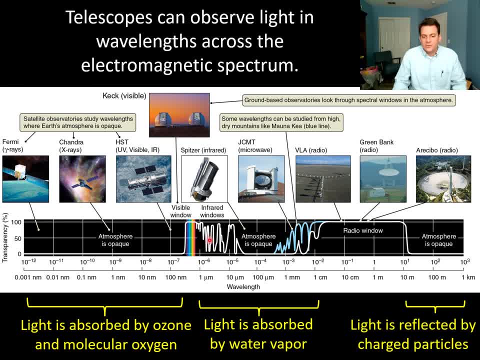 But, and you can see there's a lot of there's wiggles here. So it turns out there are some wavelengths where that the atmosphere, the atmosphere is opaque, So there's basically transparent to it, And then there are nearby wavelengths that is basically opaque to it. 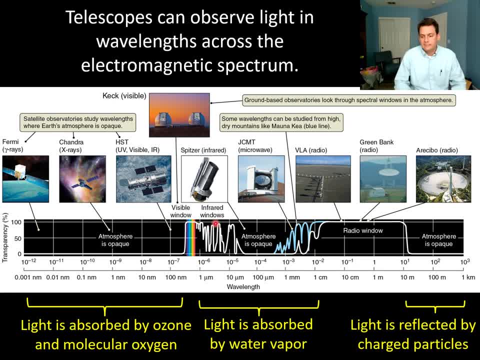 This is entirely dependent upon the electronic structure, the energy levels of the molecules in the atmosphere. So if you wanted to calculate this thing, that would be a very Herculean task involving supercomputers and so on, But it's totally determined, you know. what wavelengths get through and what wavelengths don't is just determined by the, you know, the atomic and molecular energy levels. 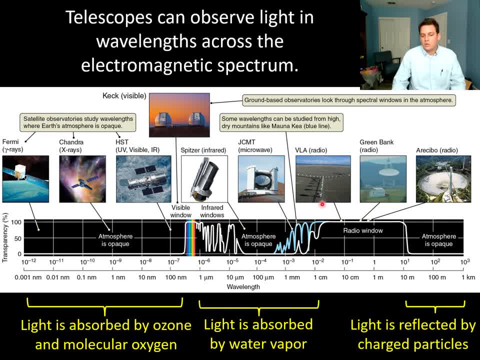 So it's completely independent of the stuff in the atmosphere. And then there's something called a. you know, there's an opaque region here where these wavelengths don't get through. There are, and then we have what's called the radio window, where radio waves are very transparent to the, or the atmosphere is very transparent to the radio waves. 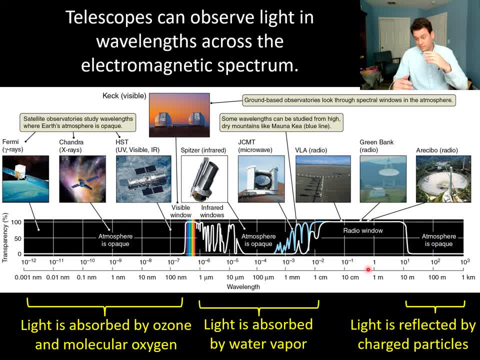 And then, finally, if you get to very, very long wavelength radio waves a little bit above 10 meters in wavelength, the atmosphere is opaque again. okay, so, so, as a result, there are some things, some wavelengths, that you can observe effectively on the earth, and there are other wavelengths that you 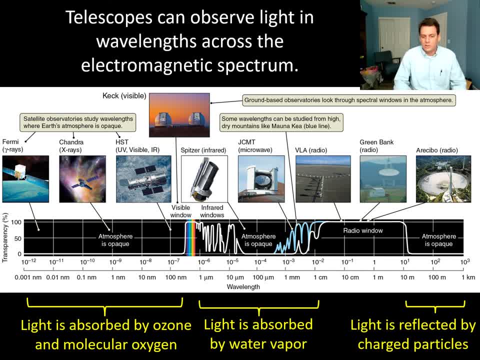 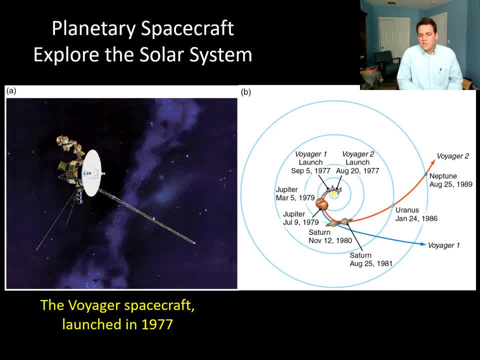 have to be out in space to observe, and so we we deal with with what we got as best we can. so we send spacecraft out and we're getting near the end here. so I'm just kind of giving you a couple of final tidbits here. the Voyager: 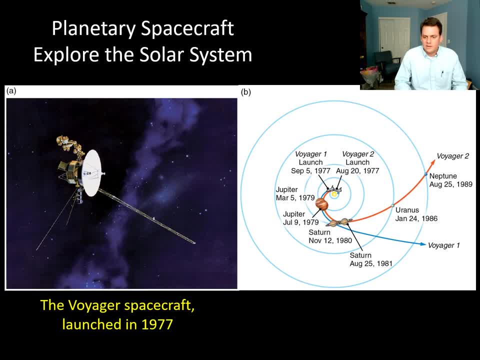 spacecraft, for example, launched in 1977. it's on its way out out of the solar system, is now out of the solar system, depending upon how you, how you define a solar system, but but it's made various observations over over decades as it, as it moved on past every planet there is. 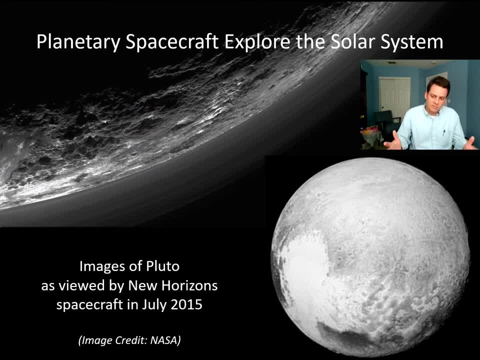 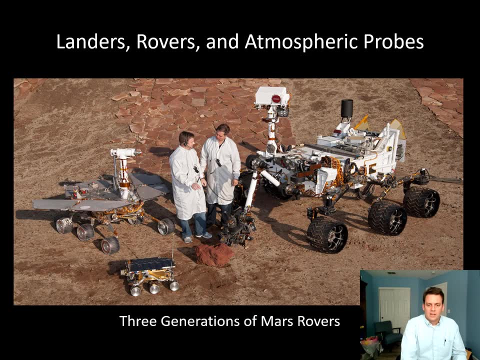 finally, I got an image of Pluto here, which is no longer a planet but still worth an image we also send. and if you're wondering what on earth any of this stuff has to do with telescopes, remember the actual title of this lecture is has to do with just the technology. you know everything that we. 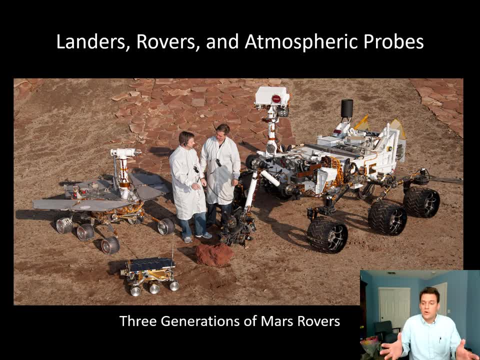 use to sort of investigate, and so most of that is telescopes, but we also have some other things. so now we have some Mars rovers that go and actually walk, or, you know, not walk but roll around on Mars and try to dig up different objects, like Earth, for example. if you've seen- that's been in the news- 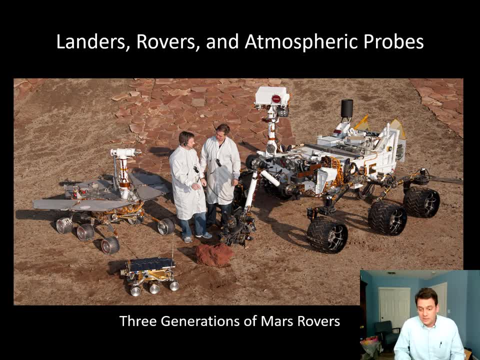 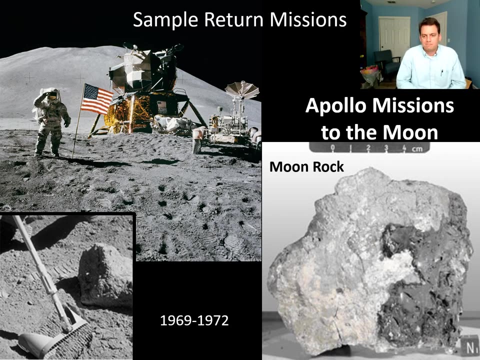 recently, and so these are things that that obviously are pretty restricted to nearby objects. it's hard to go to a star, but for the planets that are nearby we can do it. and then, finally, we do have some sample return missions, strictly restricted to the moon, because that's the only thing that has been near enough.